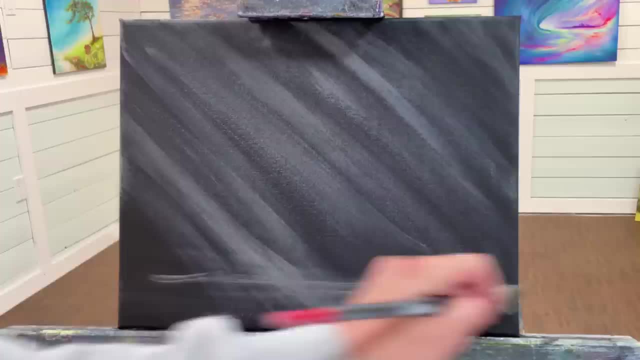 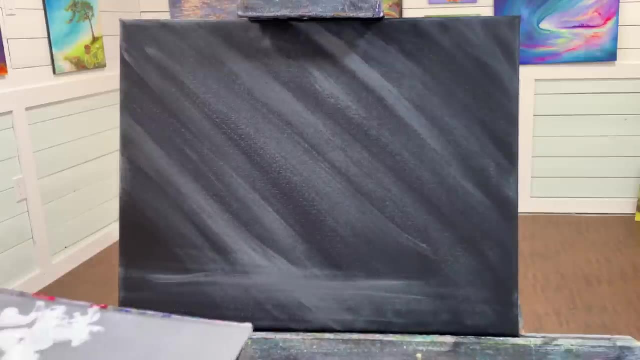 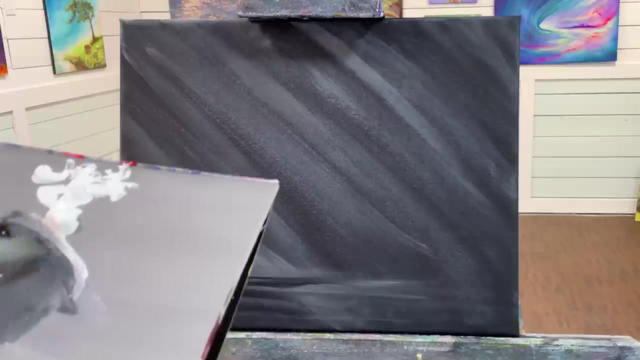 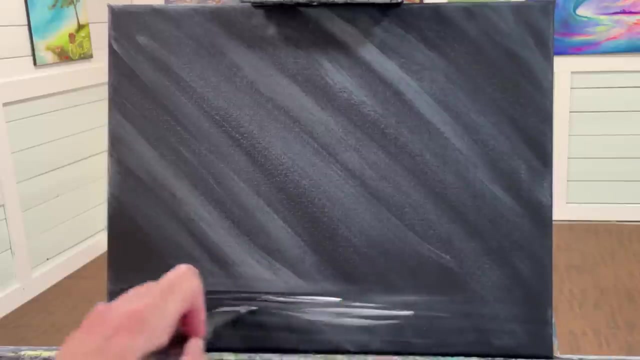 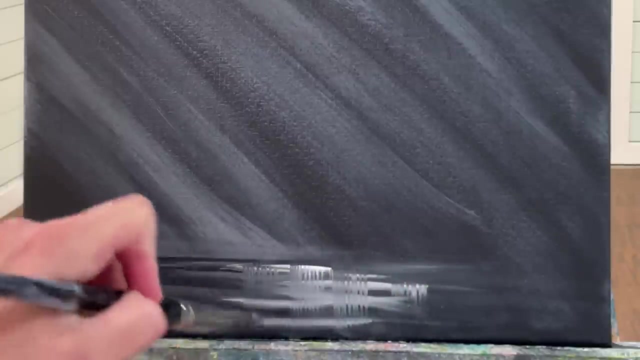 of wet floor or road or ground, Whatever she's standing on. Take a little bit of black and even just kind of create these little lines or squiggles And then a little bit more white. another tip: to make it look like it's wet or water just by pulling down or up, like this. 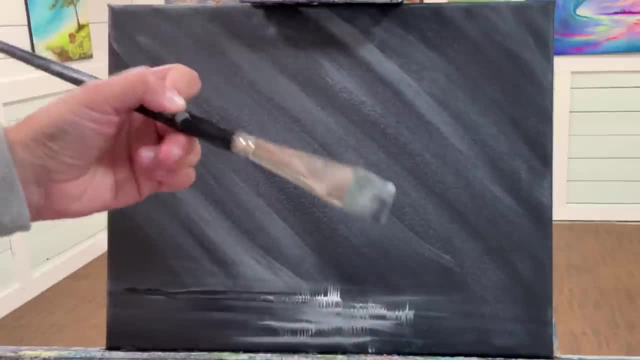 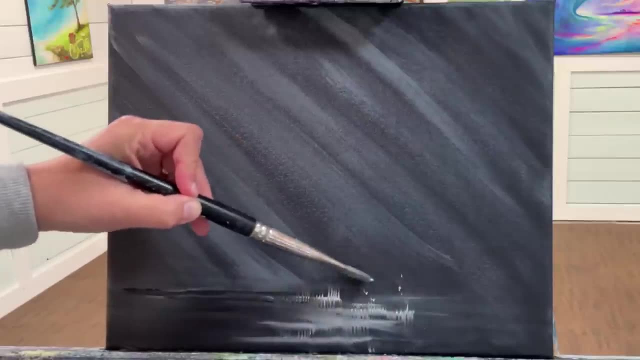 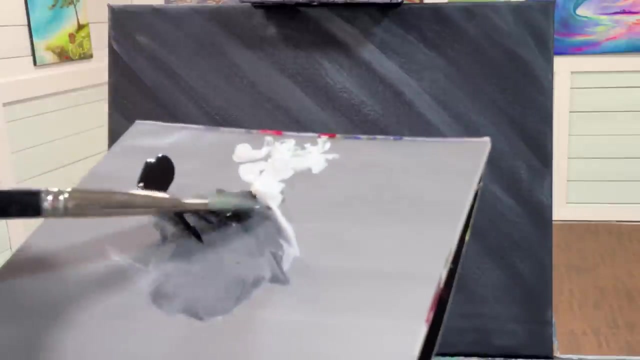 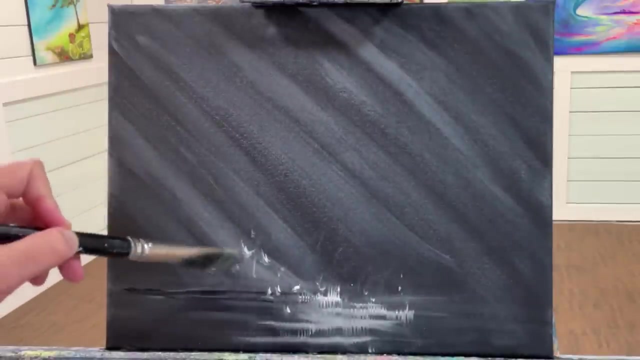 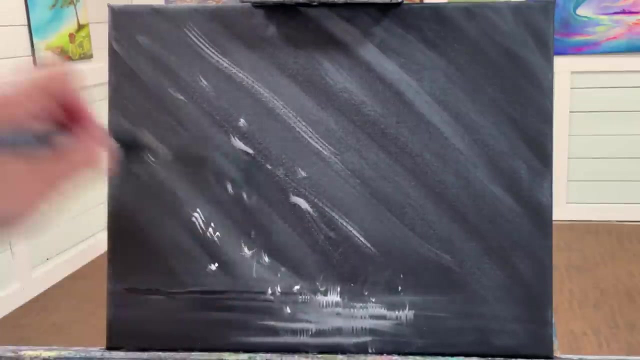 and that'll kind of look like. if we take the tip of our brush just the corner, like this a little bit of that white and gray, it'll look like raindrops and we can just continue with some little squiggles like that and then just soften brush over. 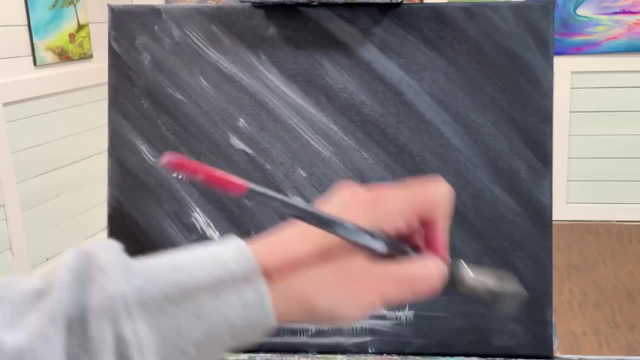 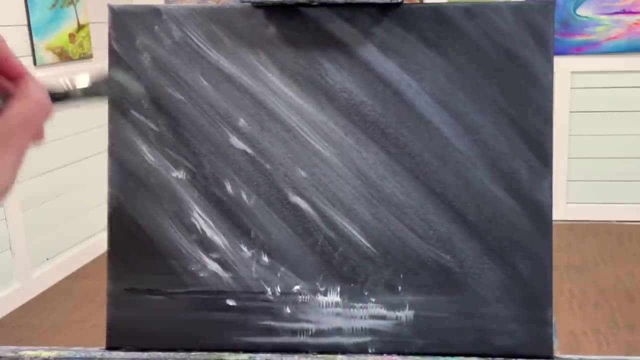 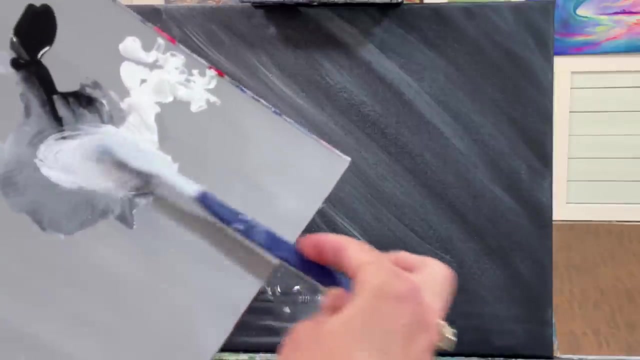 here i'm going to show you guys another tip on how to make it look like rain or snow by using a toothbrush just for crafting. what you want to do is get it wet and then just soften, brush over, just dunk it in the water and then I'm going to just scrub around scumble. 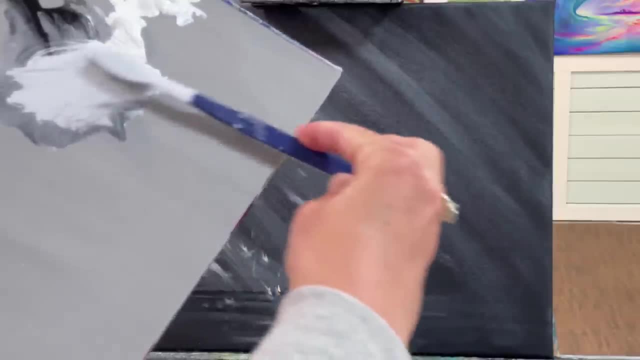 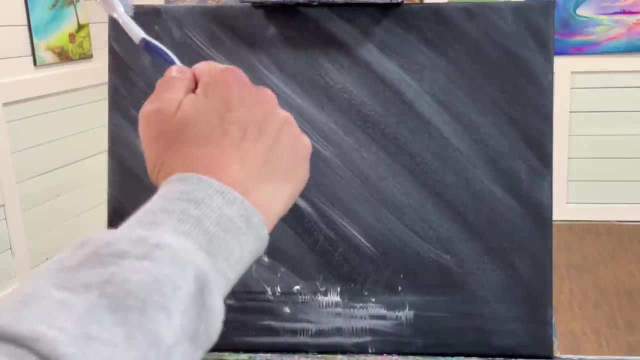 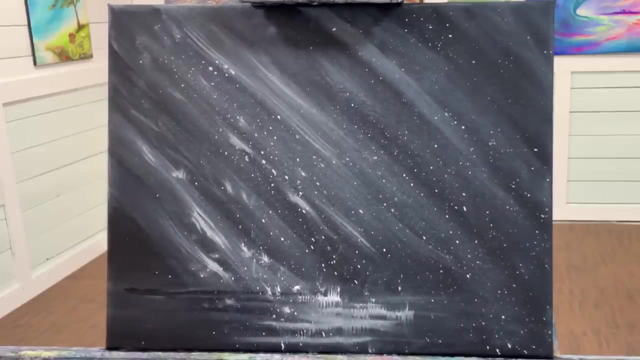 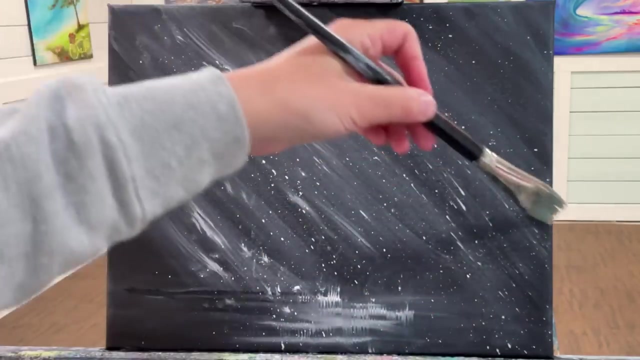 into the white paint. a little bit of gray in there is fine too. then I'm going to take my finger, hold it like this and just spray like that. I'm just going to take my brush again here, my flat one, and very lightly glide over, barely touching that canvas. 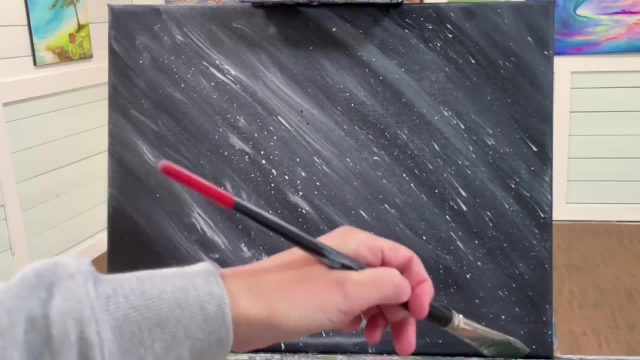 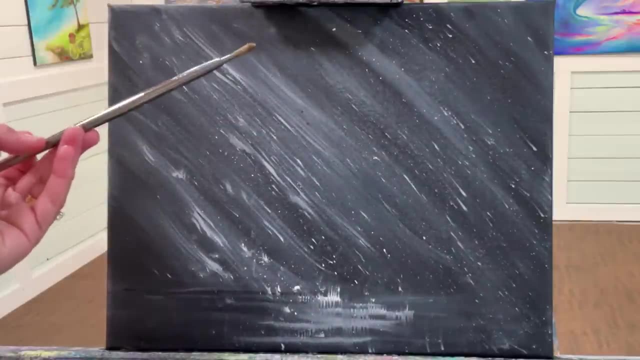 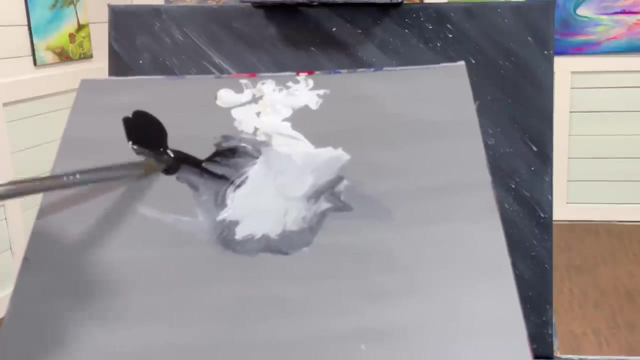 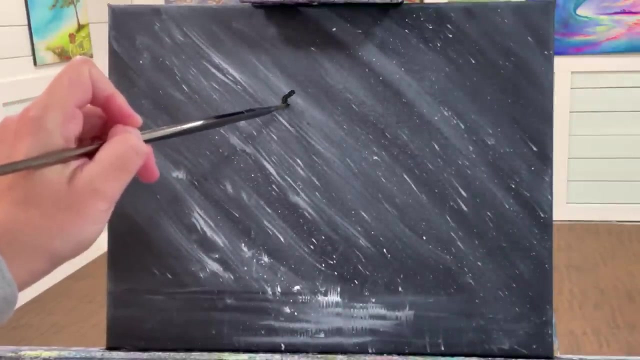 and it gives us the illusion of raindrops. to paint our lady today I'm going to be using this number four filbert brush. I'm going to take black with my filbert brush and just add a little oval here. that's a little bit bumpy. we're not going to see her facial. 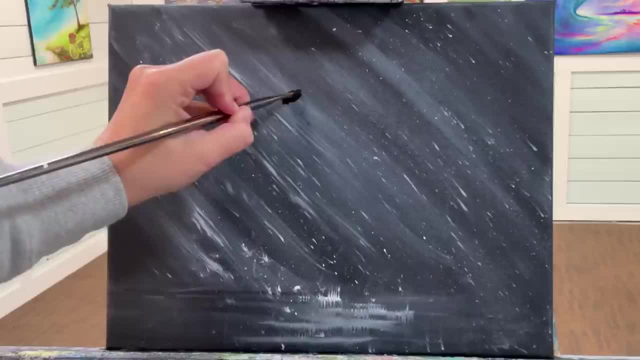 features, but we'll just see just a suggestion. so if you want to take a little bit longer for more detail on a face, you can do that. I'm just going to keep it really simple and impressionistic. so say, right, here's the forehead and a little nose. 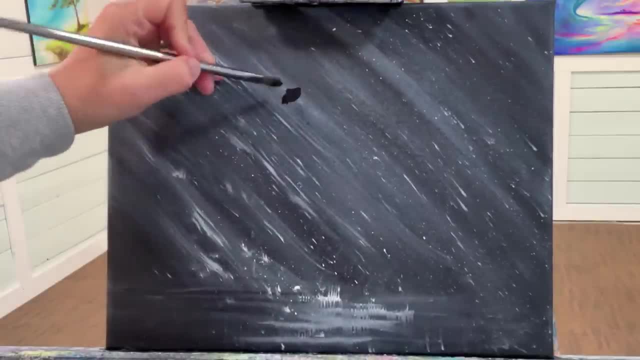 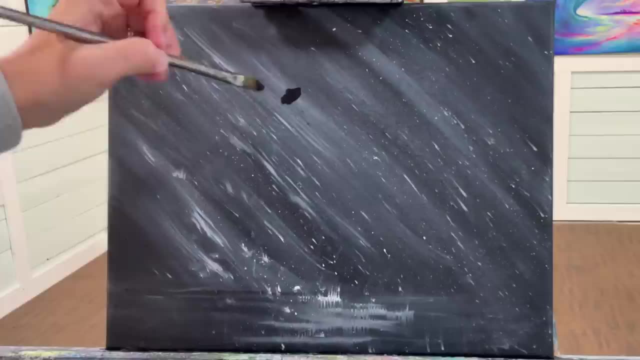 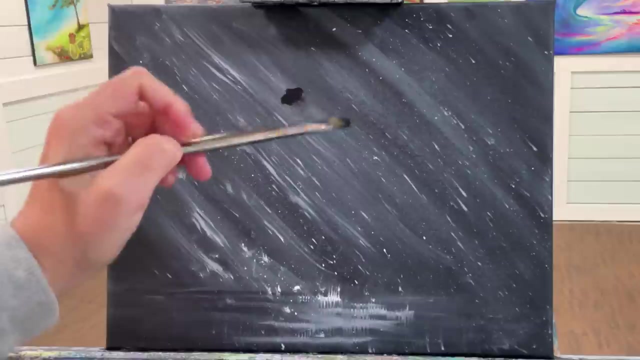 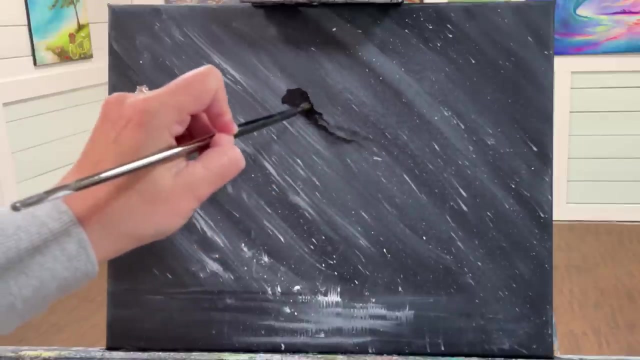 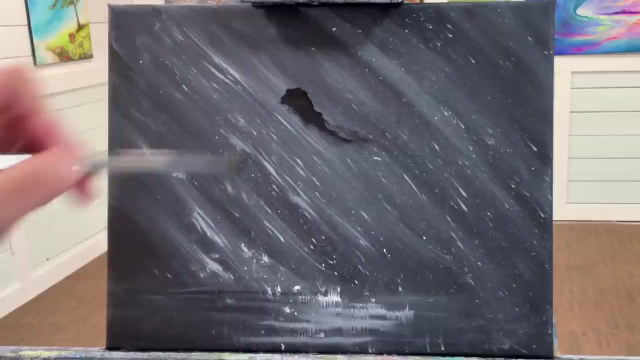 and the chin, and then I'm going to outline it a little bit later on to make it really stand out, and then we'll have her hair flowing. so again, just little wiggles here, wiggles and squiggles, and then pull and pull and pull. 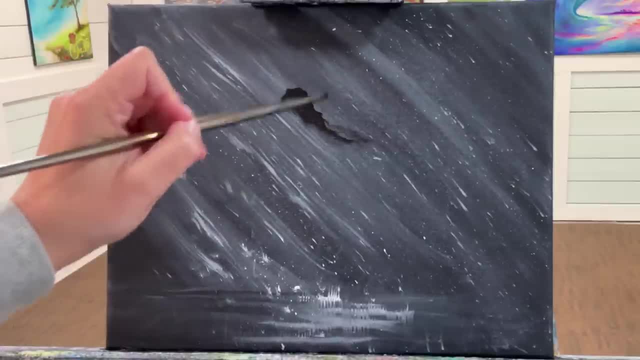 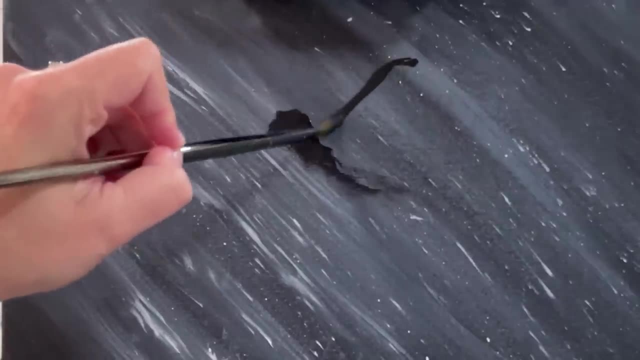 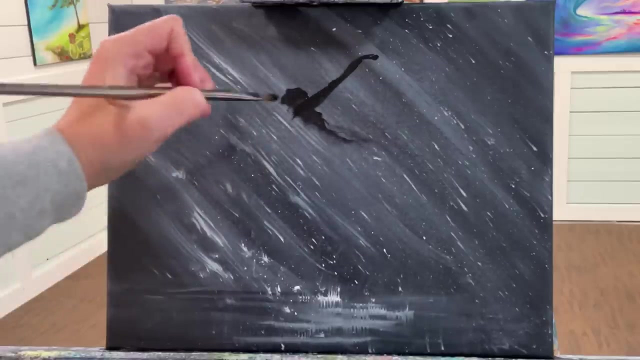 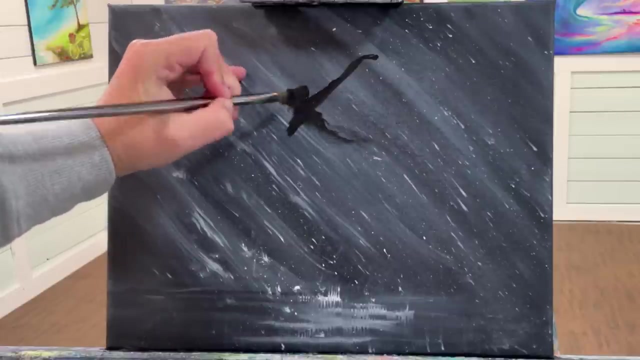 I'm going to have her arm, your hand, coming out like that, her arm and her armpit, right about here. I can bring up her, her head and her hair a little bit, and then I'm going to just bring her hair out a little bit and then I'm going to bring up her head and her hair a little bit. 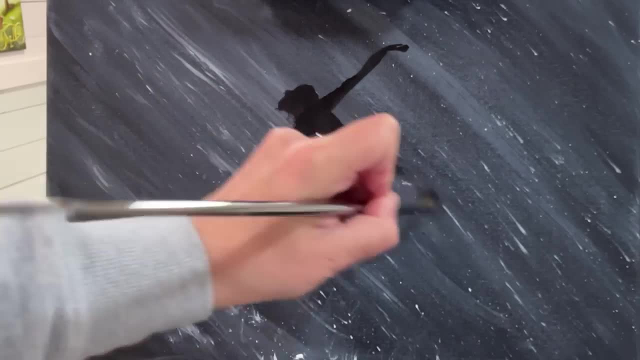 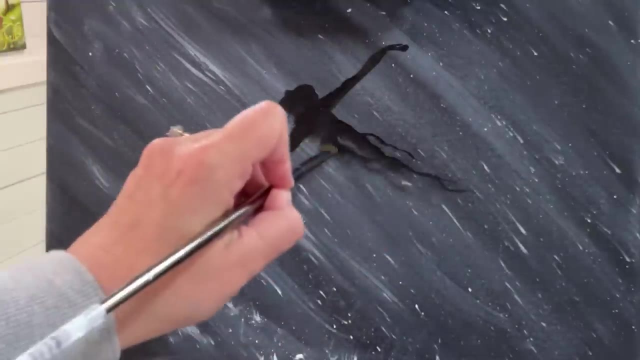 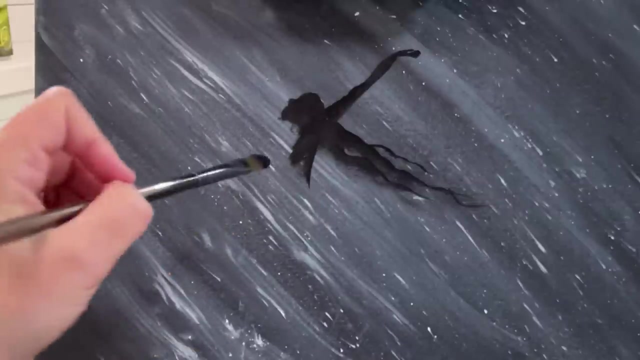 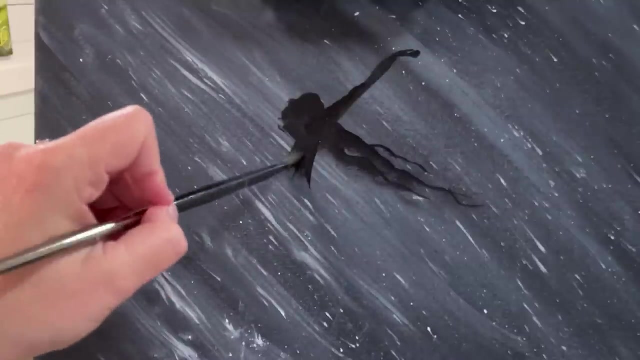 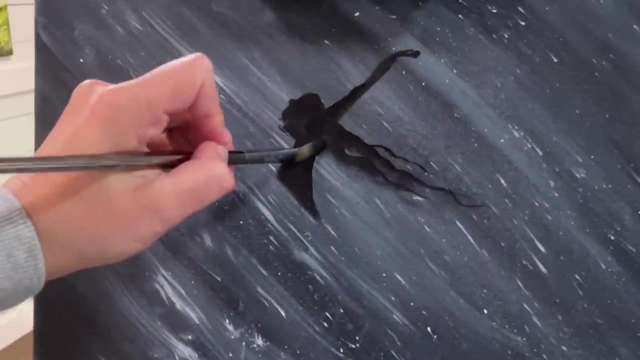 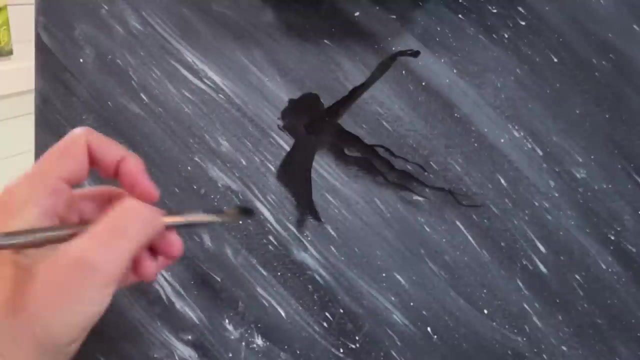 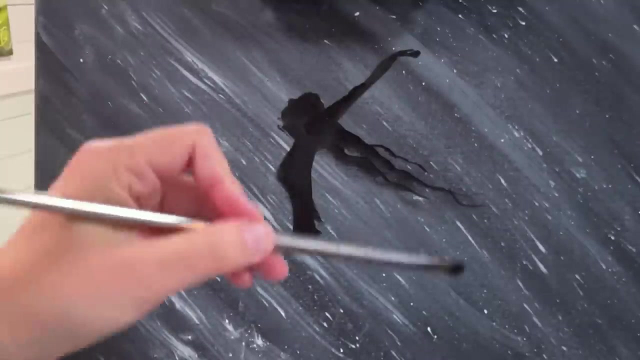 and Her neck Chest area. We're going to go in and out so we get a curve to her lower back. We want to do this in black first, so that we get a nice silhouette underneath the glowing dress that we're going to add. 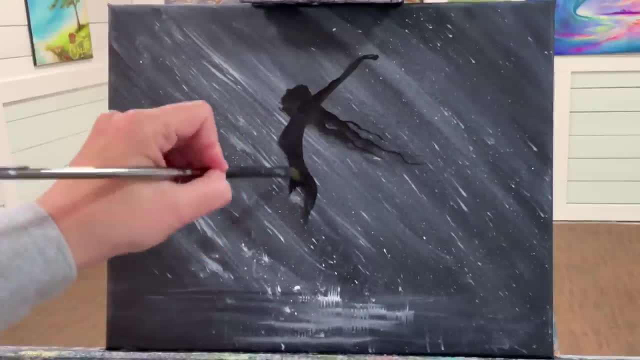 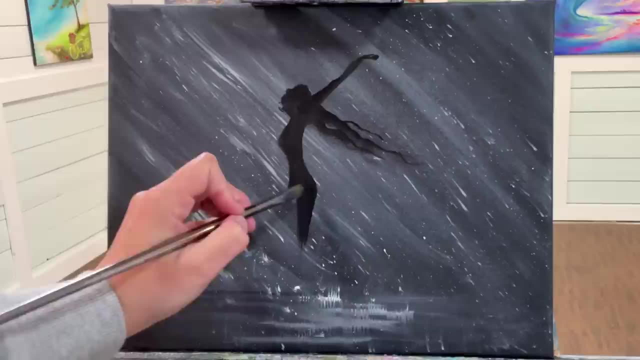 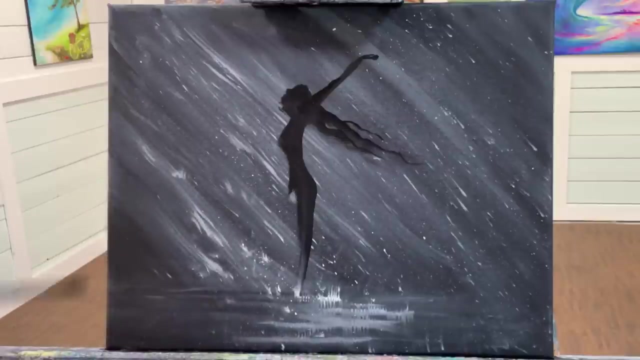 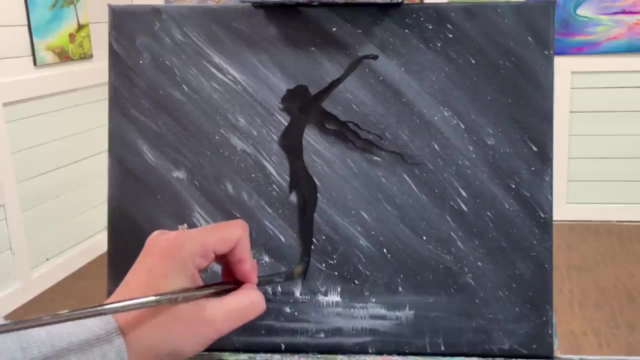 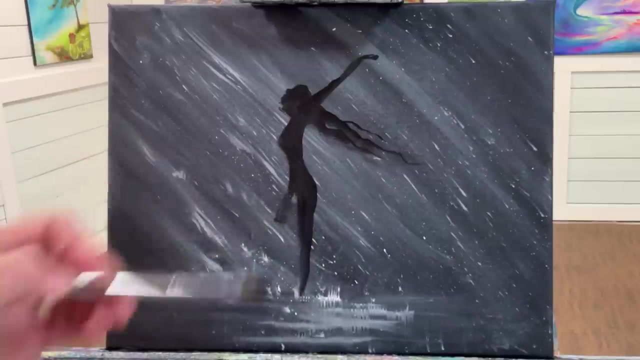 Now her bottom Eye Leg. We're not going to see too much detail, Just picked up a little bit of the rain there- Raindrops, that's okay, And her other leg is going to be coming out right about here, So we're going to bring. 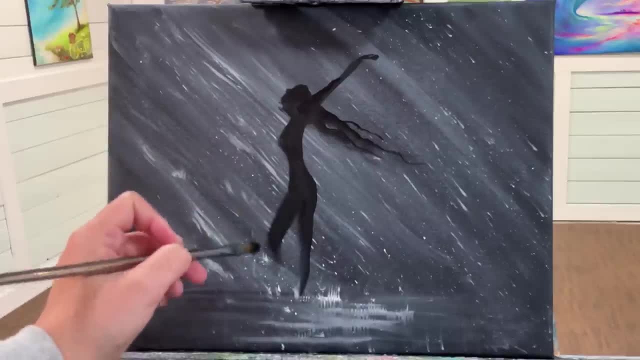 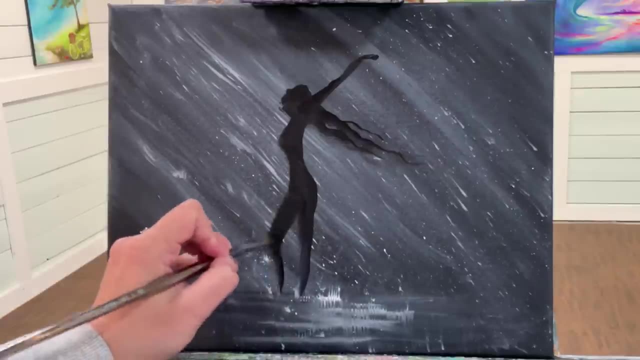 Her knee right about there And then back in and slightly Back. a little bit. Same with that one. We're not going to see her feet, But we can, if you want, just add Some black there To indicate Darker areas where her feet would be. 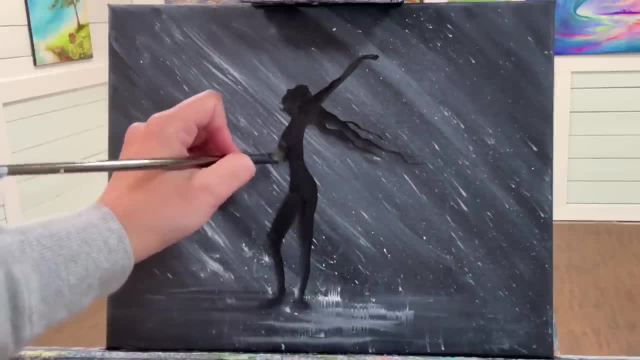 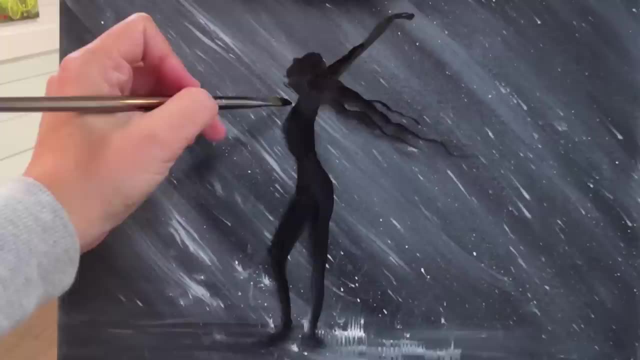 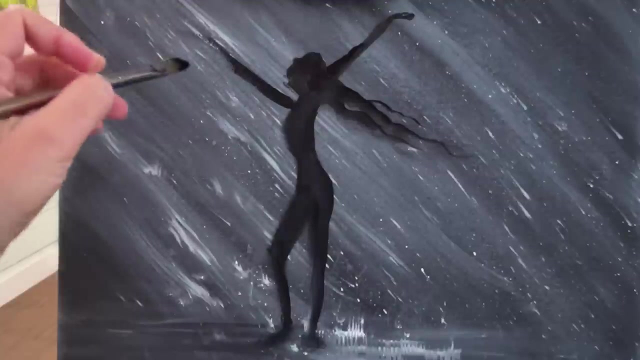 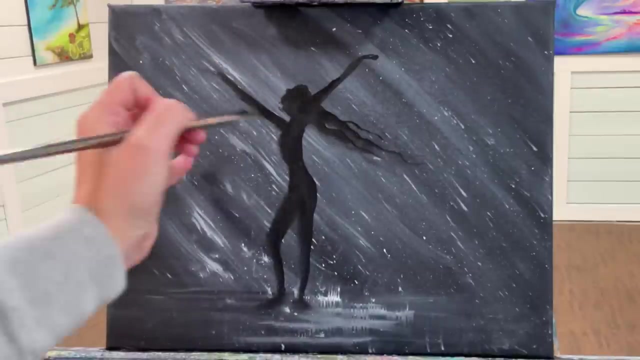 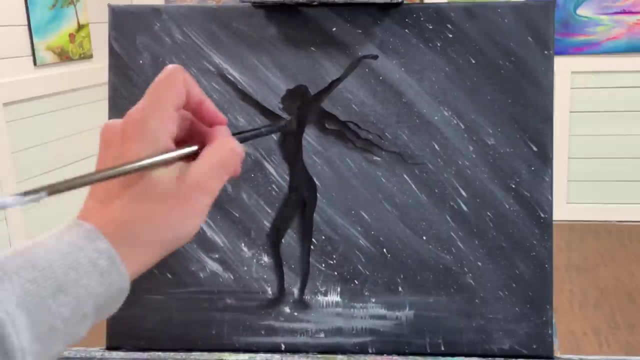 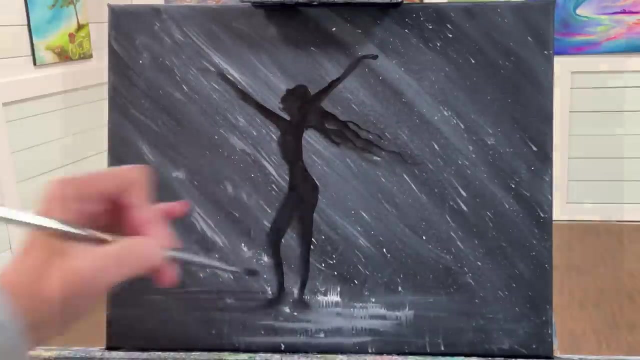 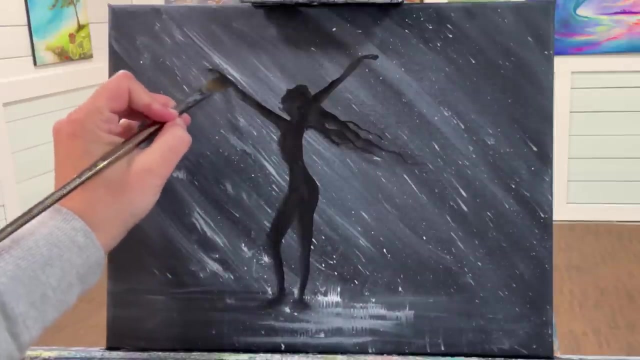 Okay, Okay, Let's see, And then we'll add her other arm Right here, Right here, And then Right. Okay, now I'm going to wash my brush off. it's still a little bit damp and I can now just. 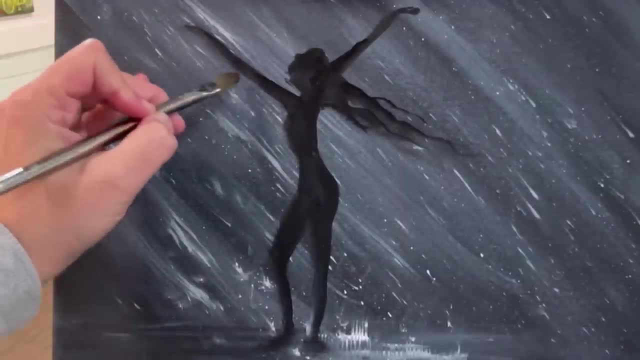 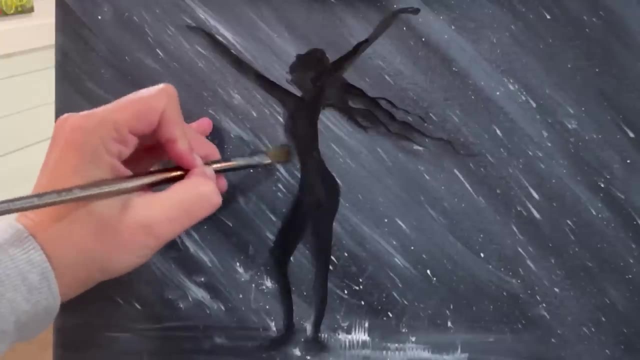 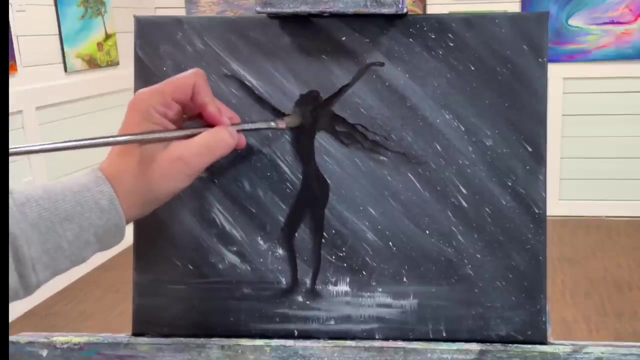 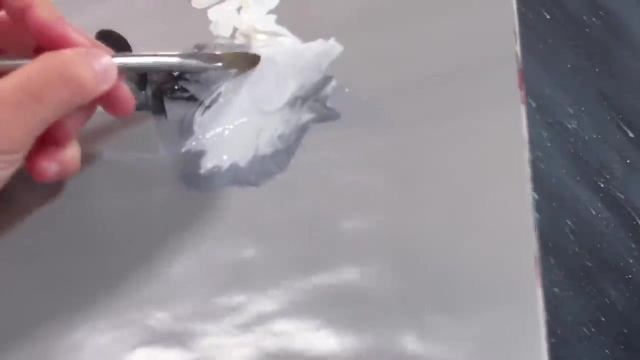 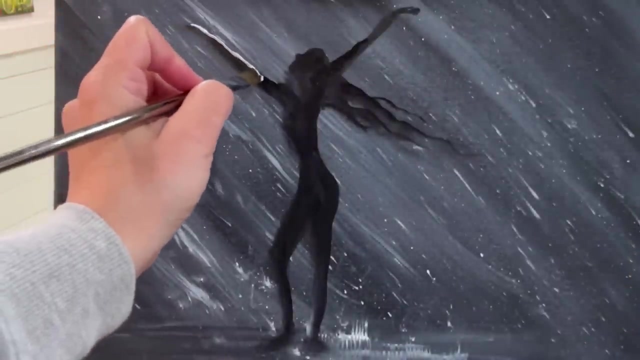 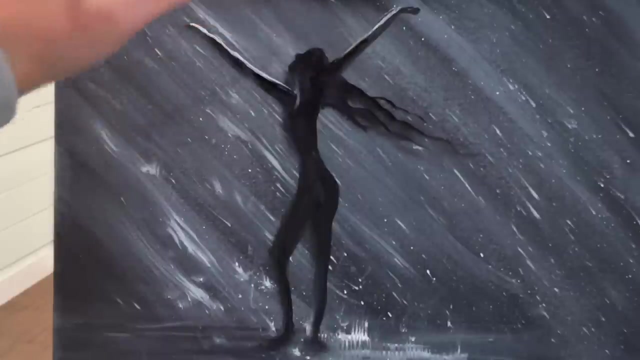 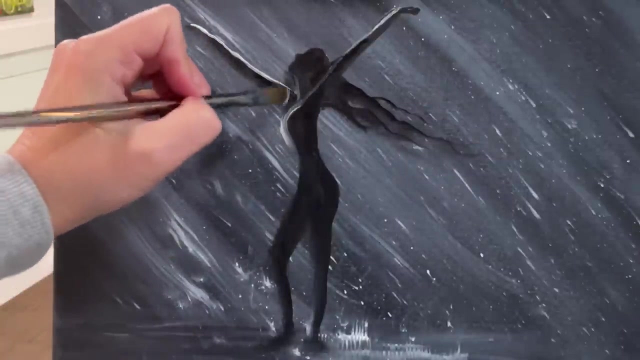 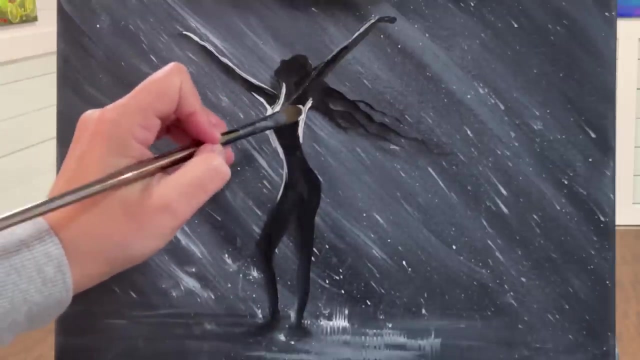 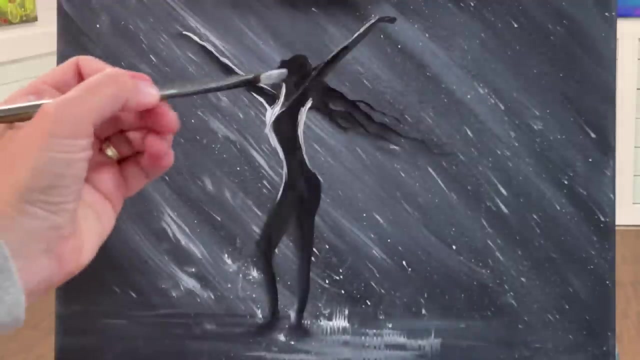 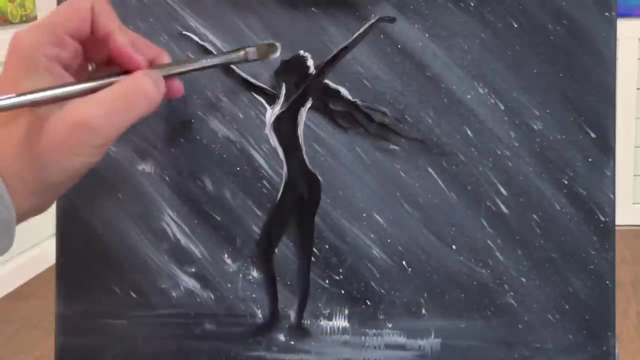 come in and take off a little bit of paint if or where I need to, And I'm going to take a bit of white now and I'm just going to start creating a little bit of a glow- Her neck, right there- And we'll add some light hitting her hair and her profile. 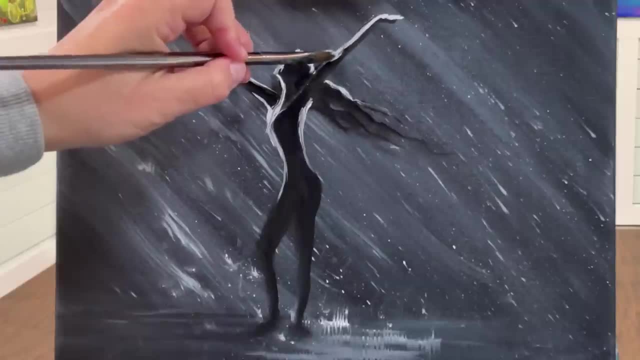 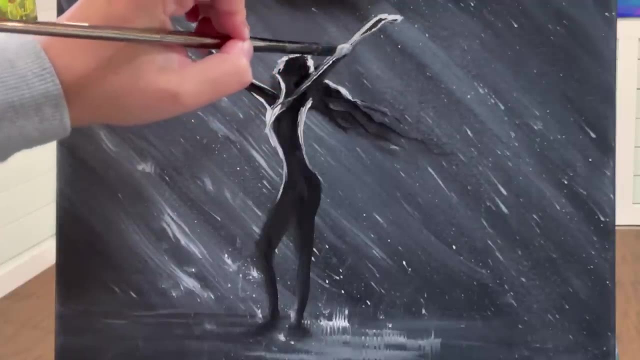 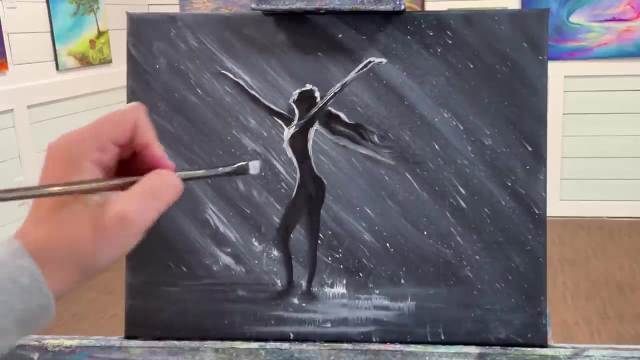 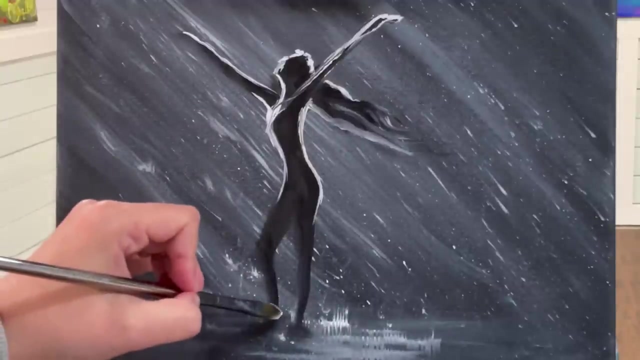 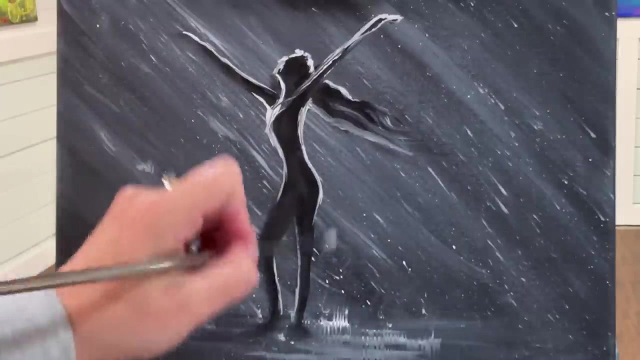 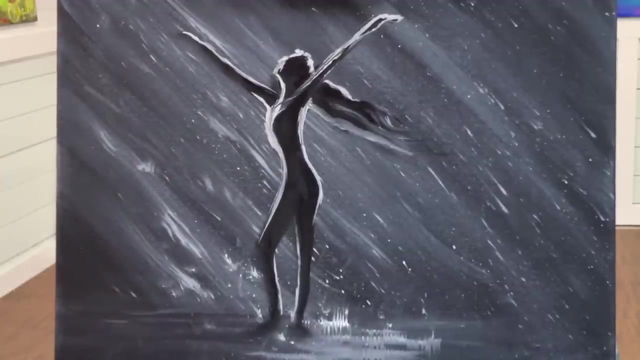 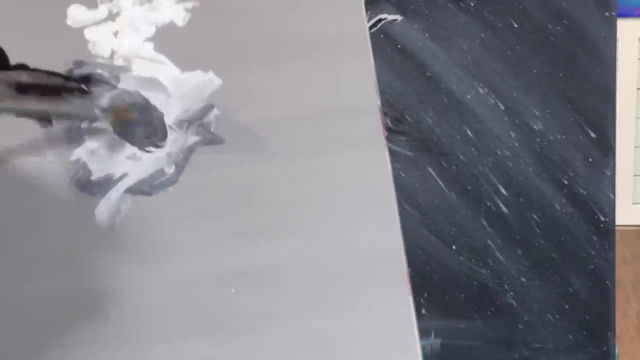 And just give her that little bit of shade. Just do a slight outline down here. Just do a slight outline down here. here, of course, we're going to have our dress. i'm going to just make a medium to dark gray color and this will be for the 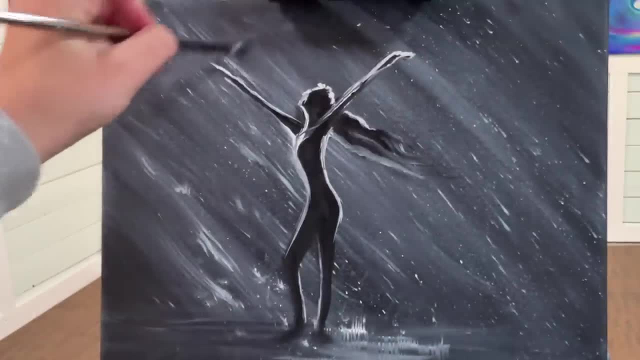 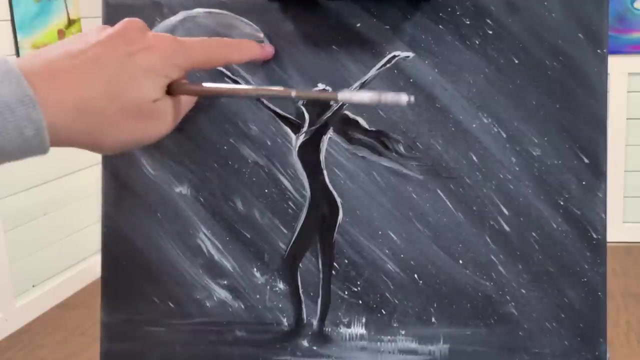 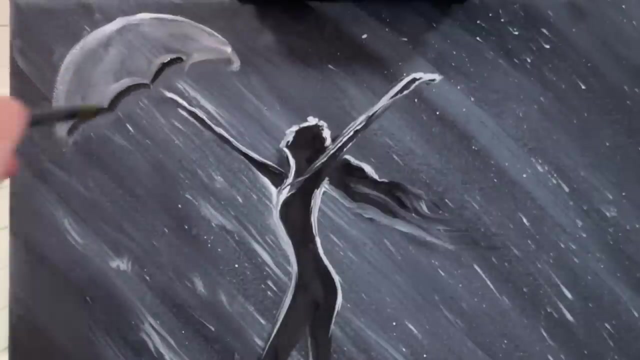 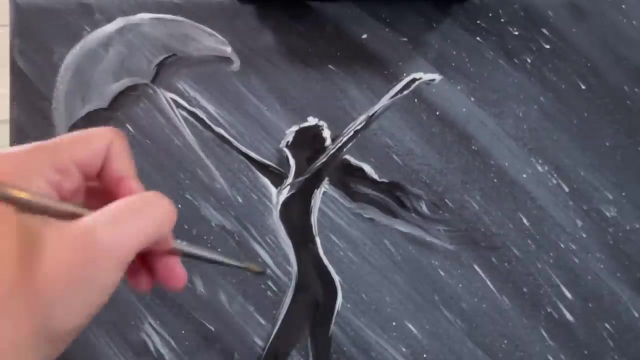 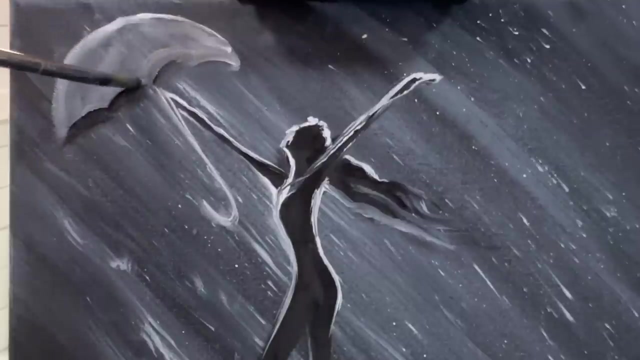 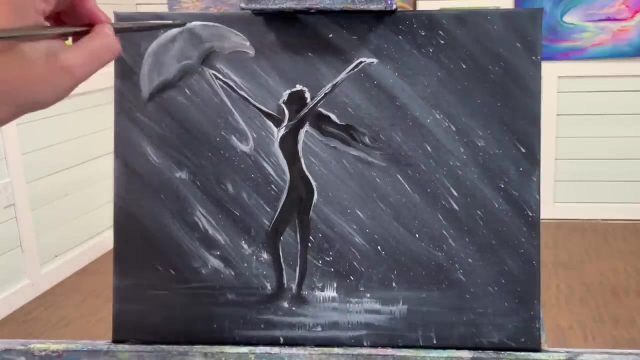 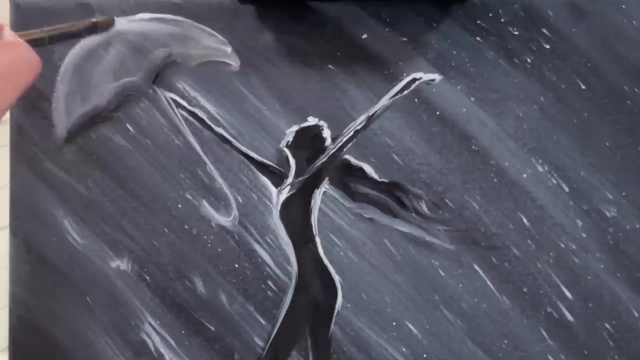 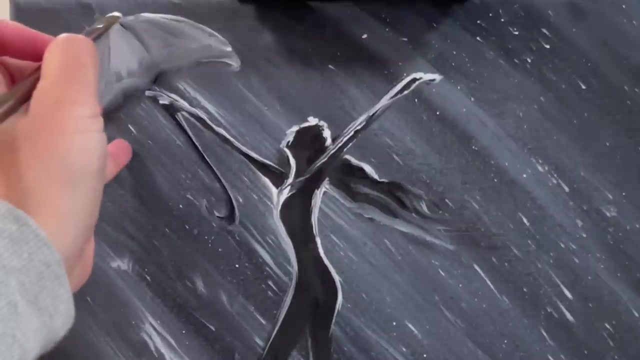 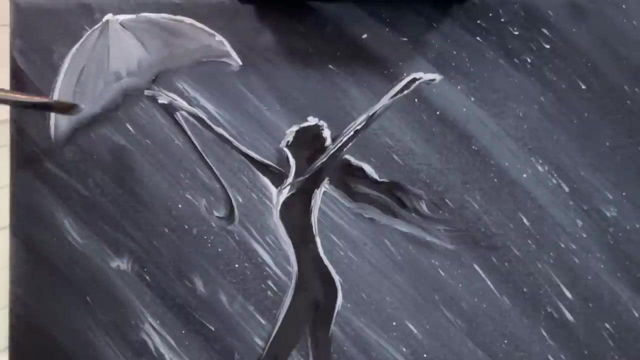 inside of her umbrella. the light will still be filtering through. so, and come underneath here, black, so, so, so highlight the top, start from this point up here, then take a little bit of black and just inside the handle, and we can outline like this: so i'm going to take a little bit of this white here. 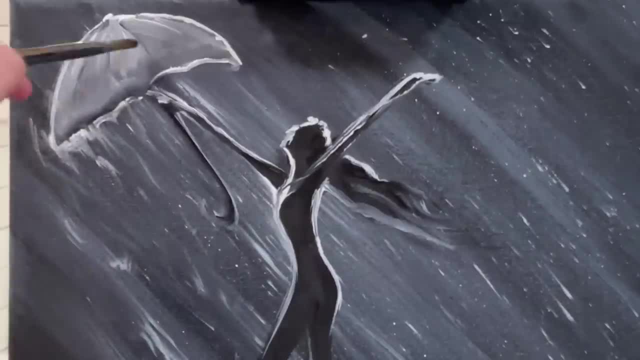 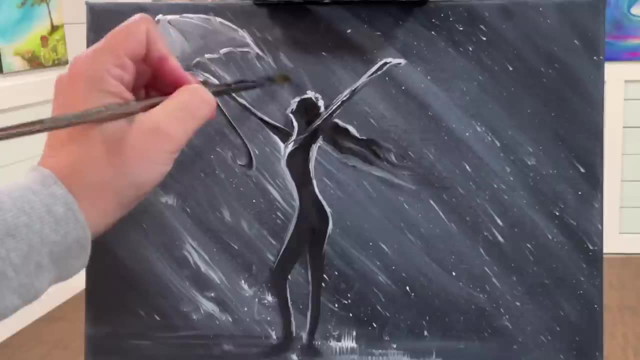 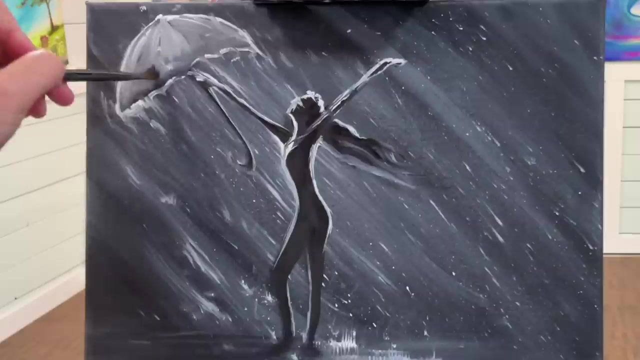 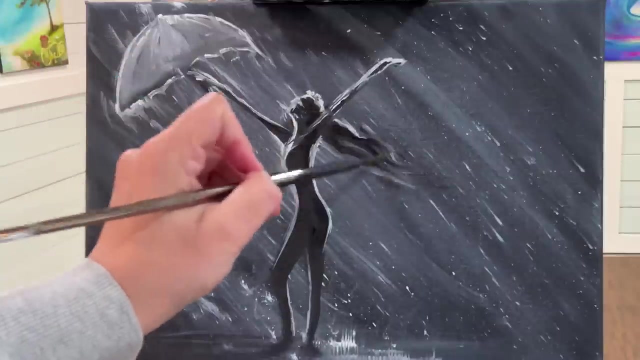 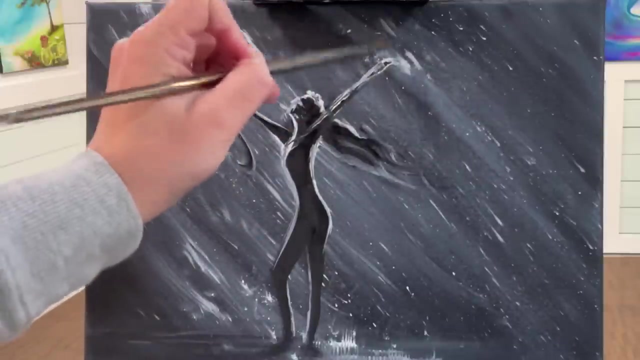 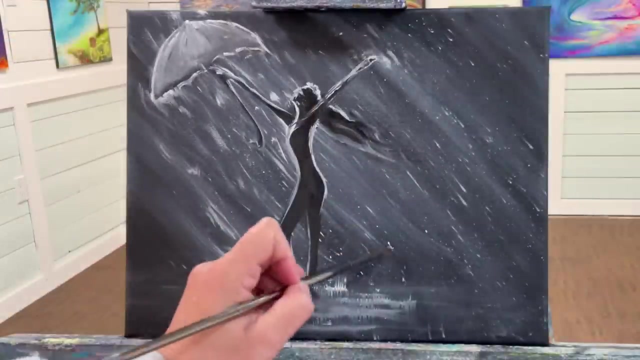 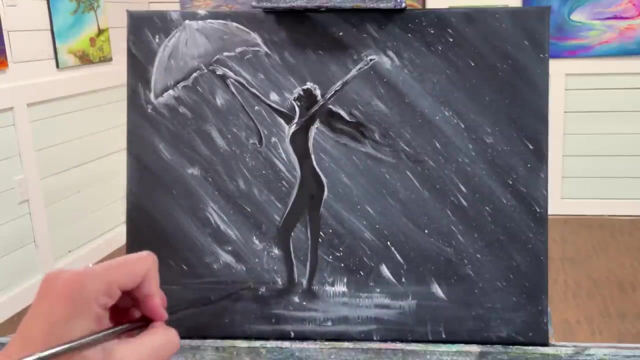 and just use it to go over the umbrella, just taking off the existing wet paint to make it look like rain. this is going to give it a really loose and natural look to your painting. so and then, if you want it to look like there's a little bit more going on, 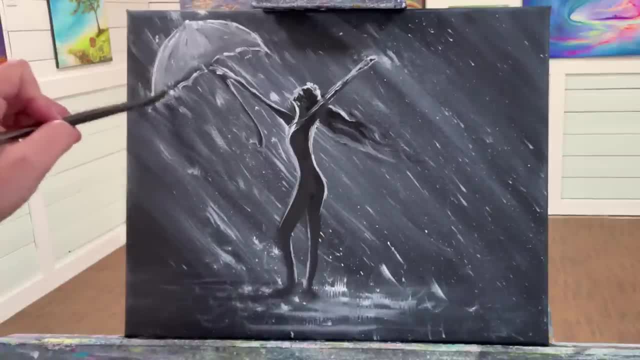 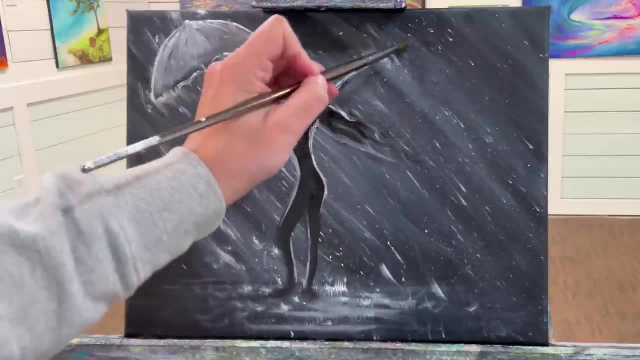 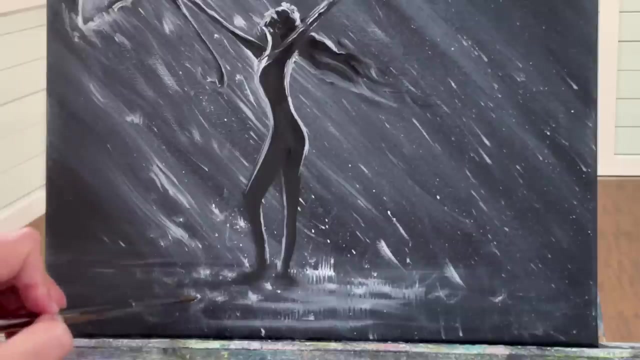 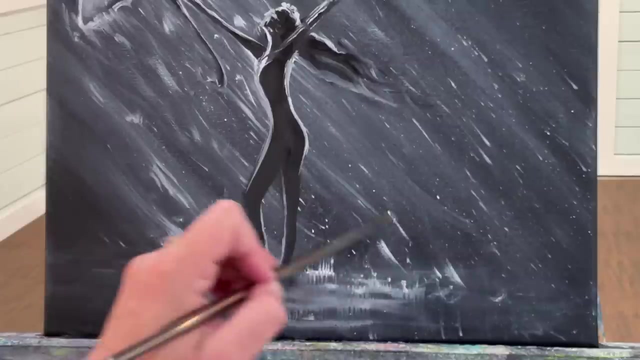 like she's sort of dancing in the rain and there's little splashes. we are going to be adding the dress in here, of course, and so we can continue that later on, but that's all you would simply do is just add these little taps and flicks. it's really that simple. don't make things harder and over complicated. 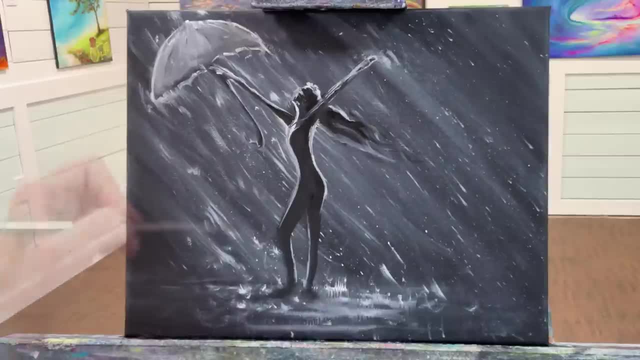 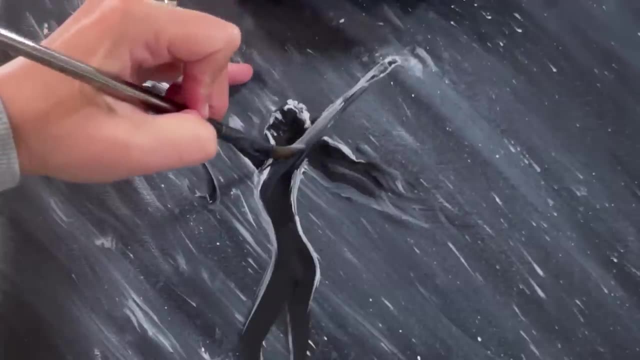 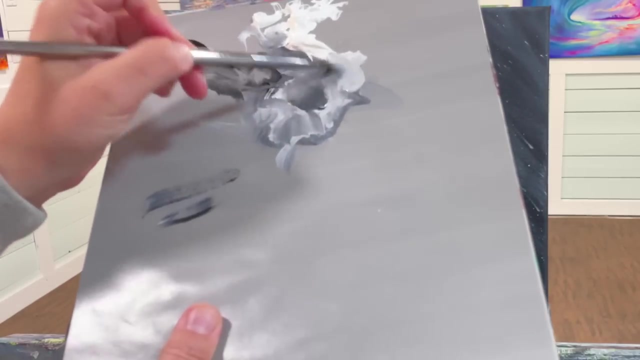 and we're going to go ahead and add a little bit of a lighter gray just to make her arm be more in front and stand out, and then we're going to continue with that light gray, picking up just a little bit more white there. so i have more to work with. 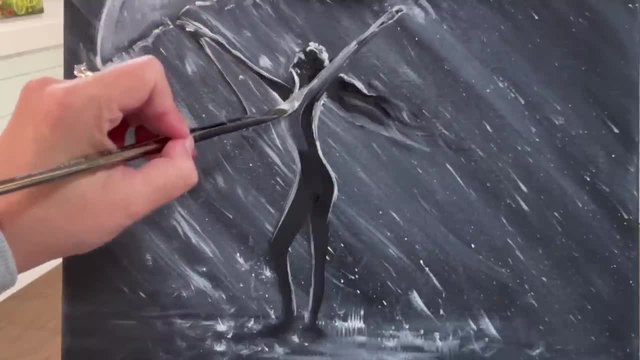 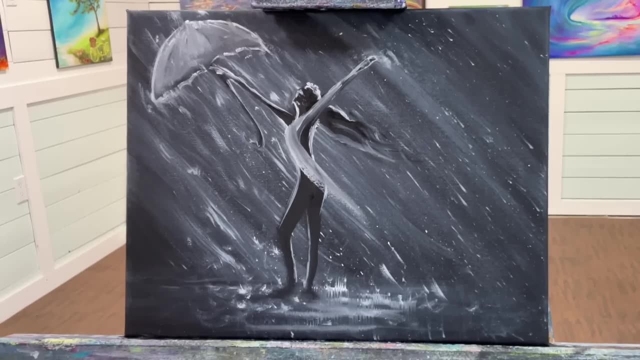 and we're gonna line it up, pull and swing over and start on her dress. what i want to do is add a little bit more water and white now, so it's kind of it's not dripping but it's very loose to work with, so i can get more of a transparent glow to her dress. 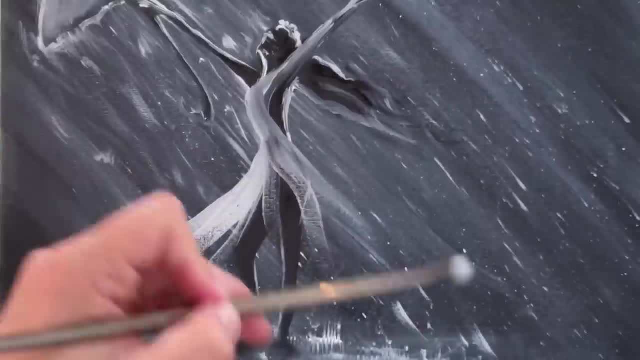 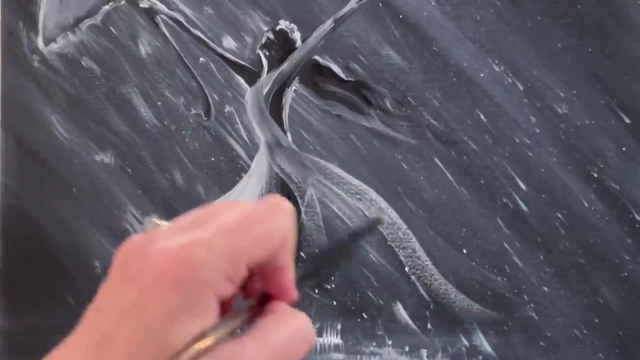 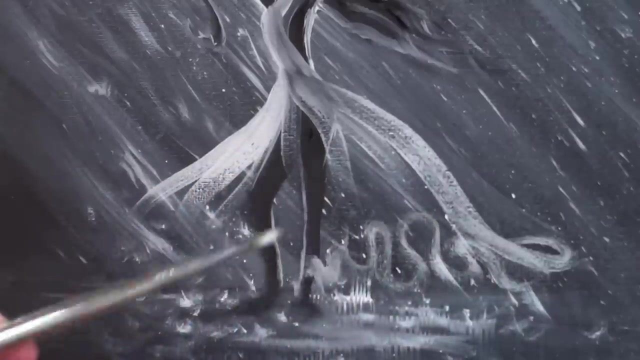 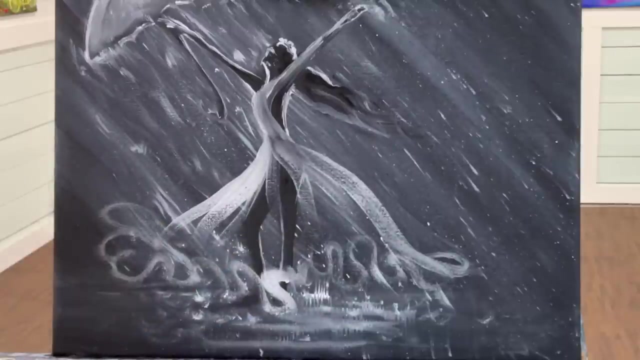 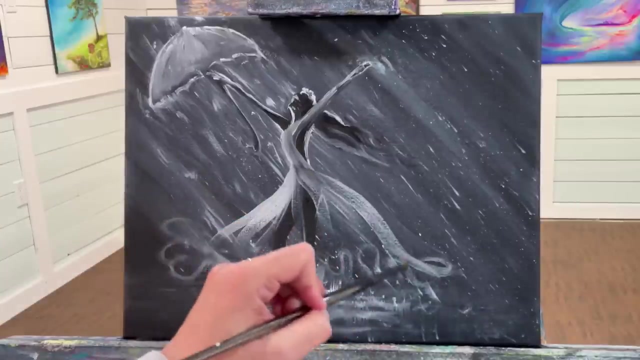 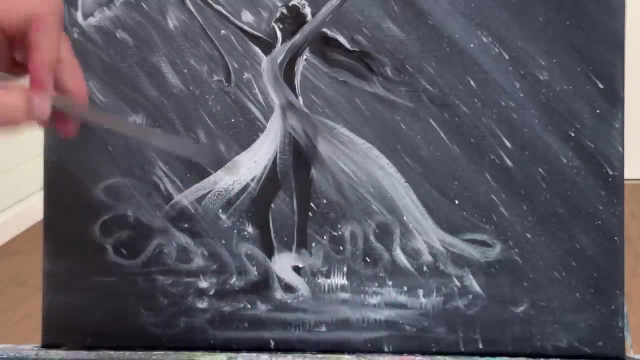 so we're going to pull these lines in here. those will be the, the fabric twisting and flowing around, and then, wherever you want to have pretty ripples, ruffles in her dress, you can just create those squiggles like that. i'm just loosening some of this paint up. 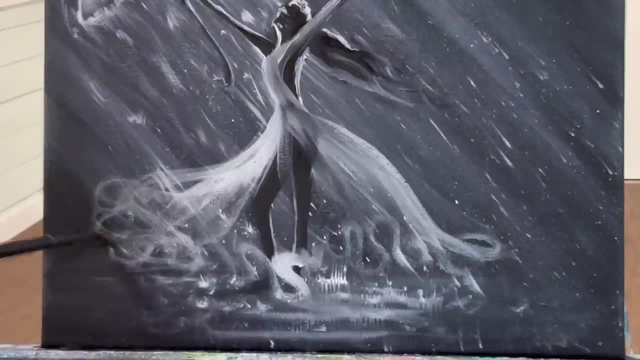 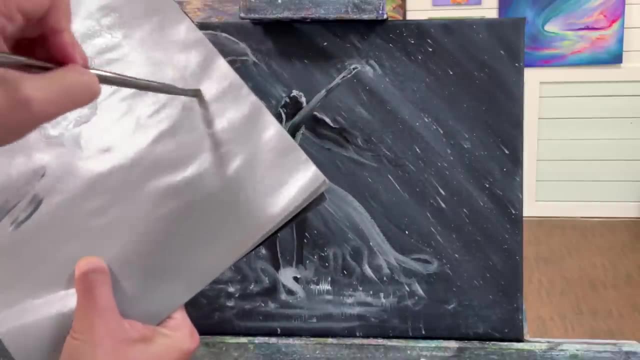 so if you're not sure how to create those, that squiggle kind of a look, it's really just about creating figure eights. so just practice, travel around while you're making figure eights and there you'll have a ruffle, bottom ruffle, and then we're going to go ahead and add a little bit. 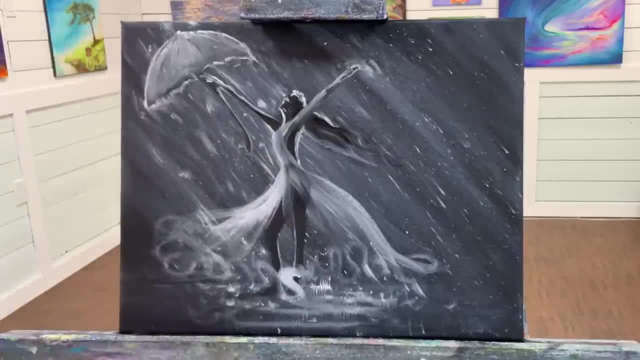 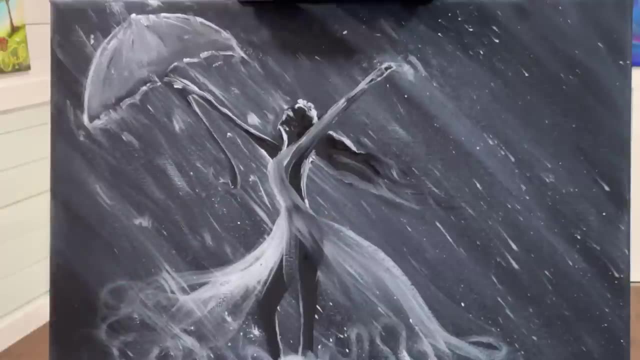 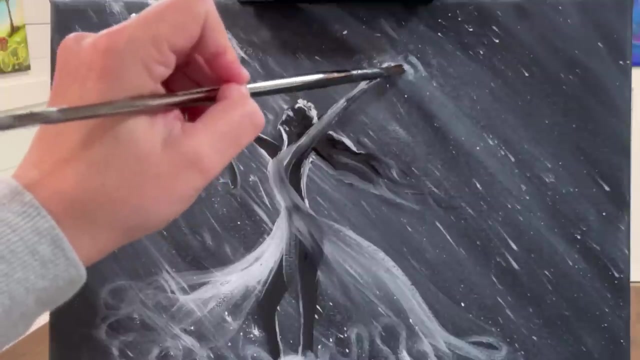 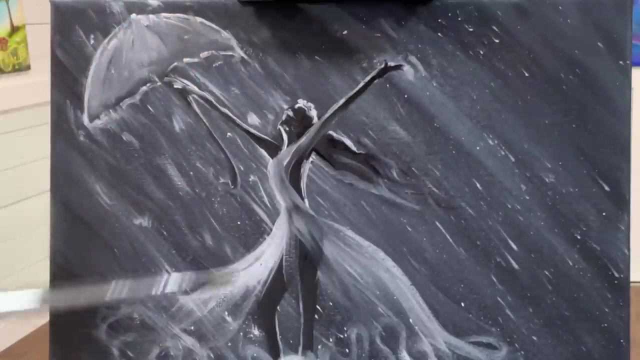 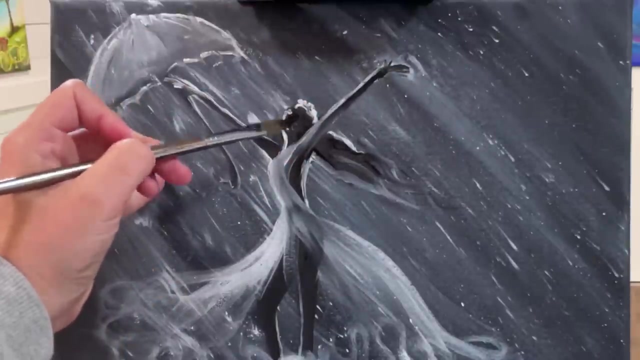 of white to the bottom of the dress, fluffy looking dress. i want to add a little bit more to her hair, make this- the hair stand out a little bit more here and just come inside, inside her arm a little bit there. i'm just going to layer it on top. so now i'm going to keep getting this. 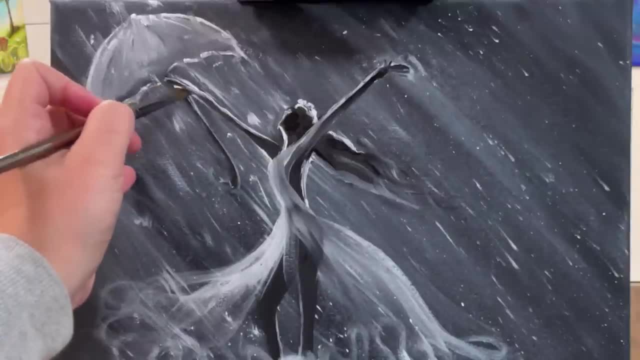 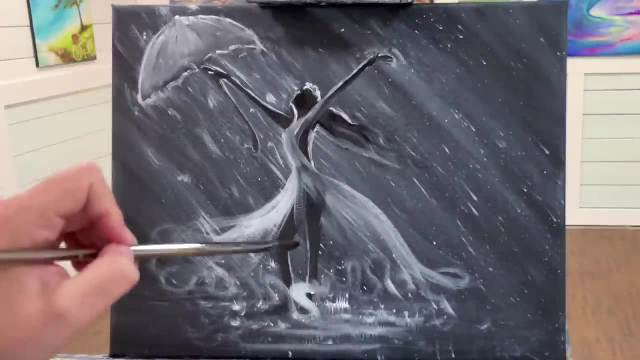 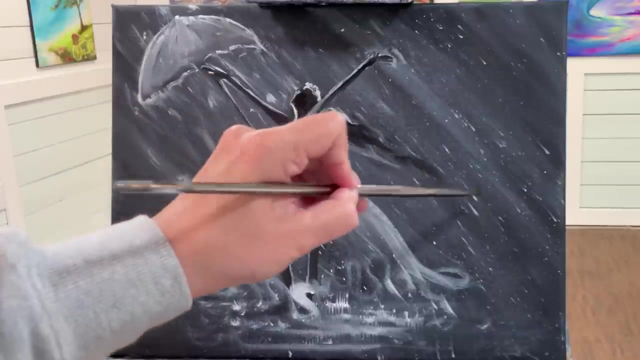 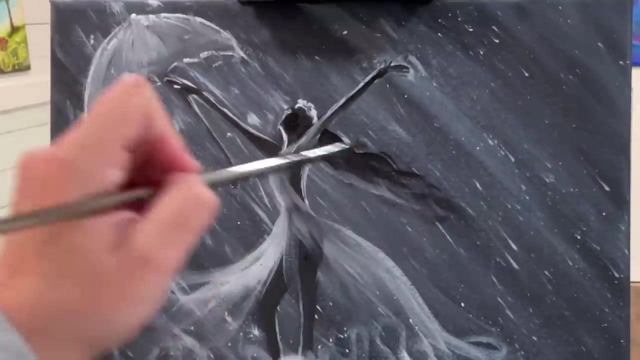 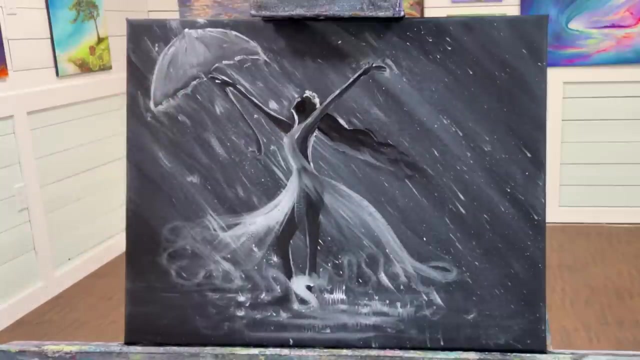 clean. it's going to look a little bit wetter and it's a little bit more fluffy in the shape of your hand. okay, so you're going to take a look at the face of theちょっと: one, two, three, four, five, six. you might recognize this, this figure, from my lady in red painting that I did. 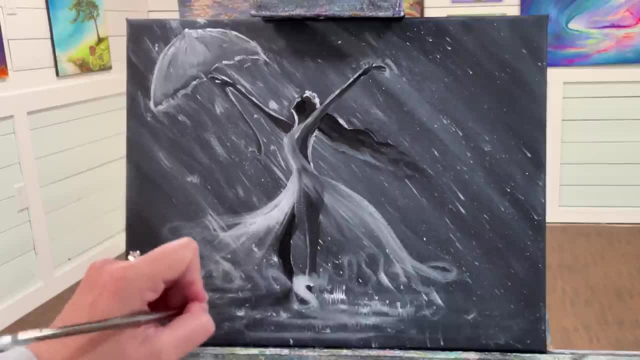 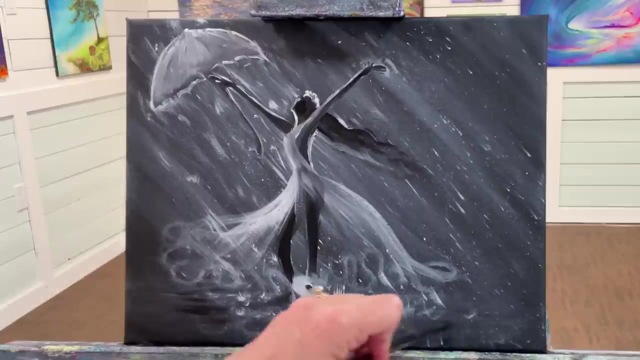 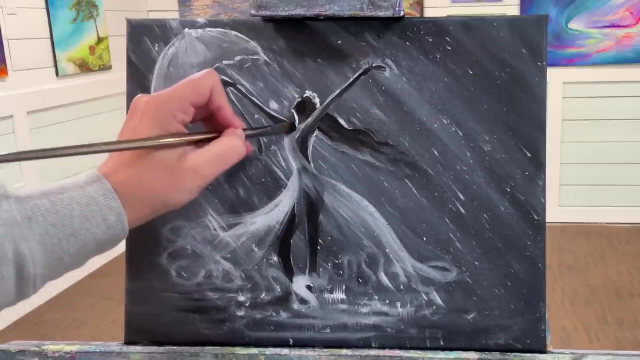 and that one was very popular and still is very popular and I think it's because she just has such a powerful pose and energy about her and people are. you guys are really loving to paint that, so I thought I would use that again. it's gonna add a little, just a little line there. 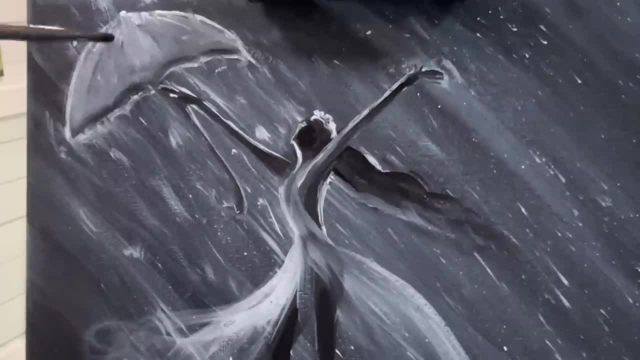 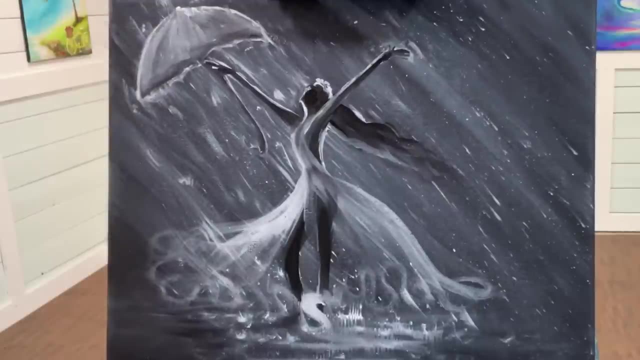 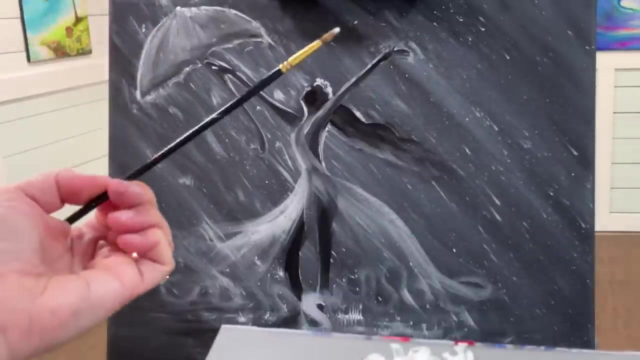 and then just add a little bit of a shadow back there, again just taking my little round brush. here come in with my white. I'm using a round brush because I can have more control with it. for smaller areas and tighter places I need to get in. so this is a. 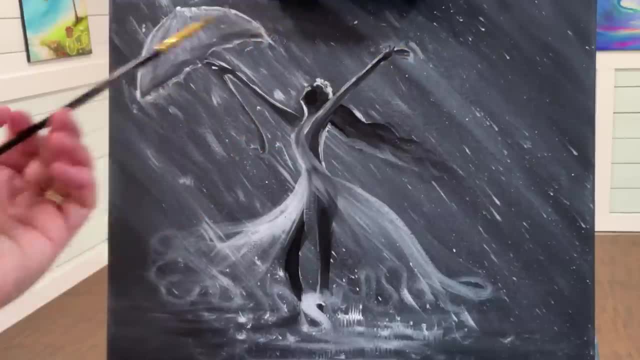 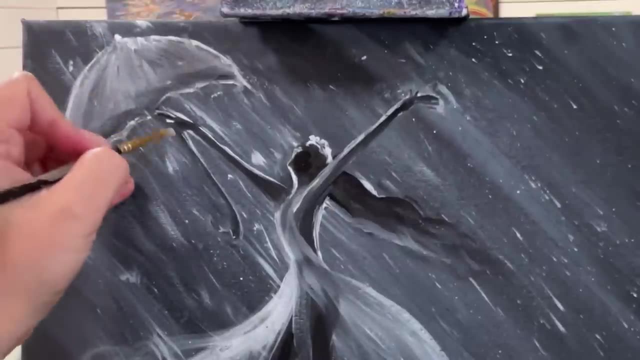 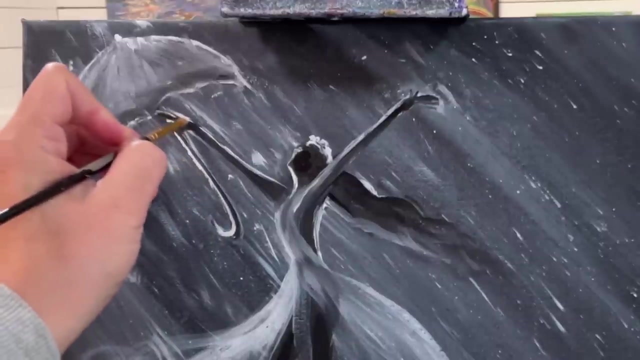 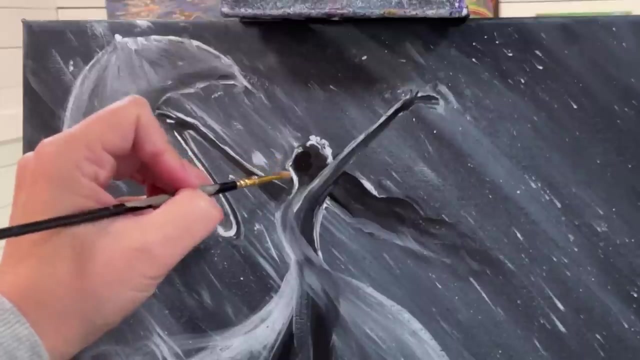 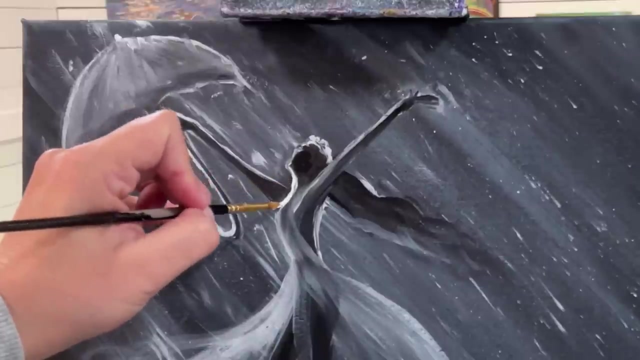 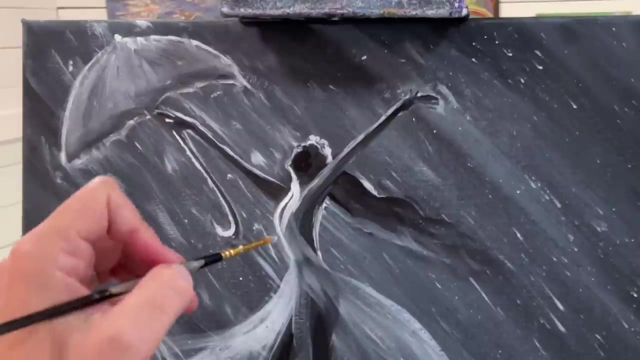 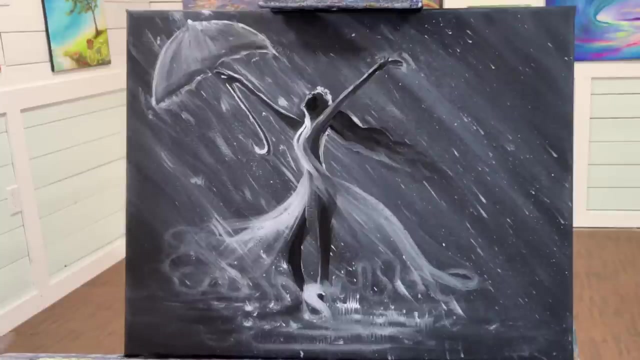 number two and there's no make on this brush. I just got a huge set from Amazon a couple years ago. it's lasted me a really long time. just outline lightly here you, And this is going to be my little window onto the wall, and this choice is quite cute. 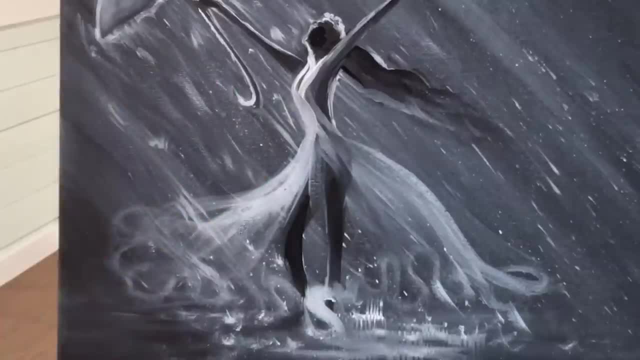 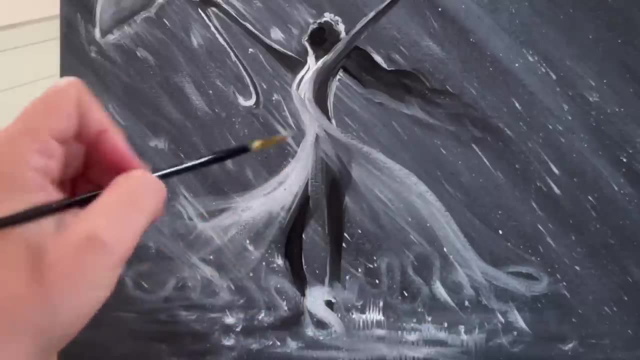 you can see it was a vaccumucha yesterday so it's going to be a grown sleeve because I originally- strange But closed- already shown other things. this Our heart like a tree. I don't like it. Your on the guy years ago and took up a little bit more time to, because I love 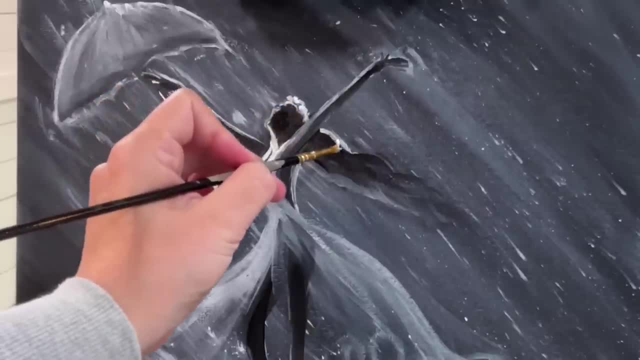 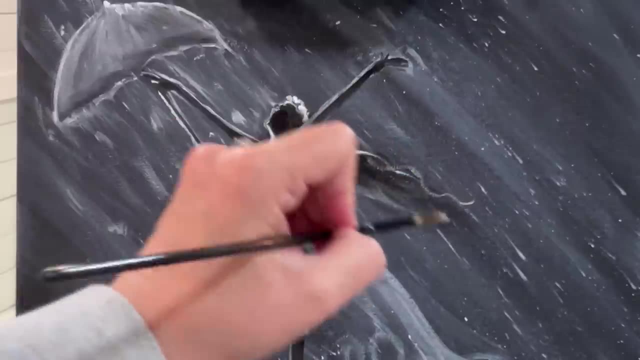 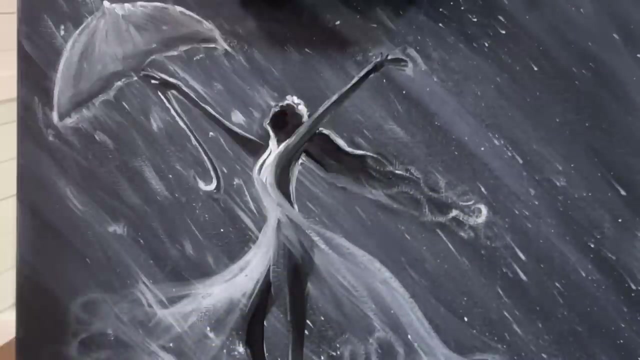 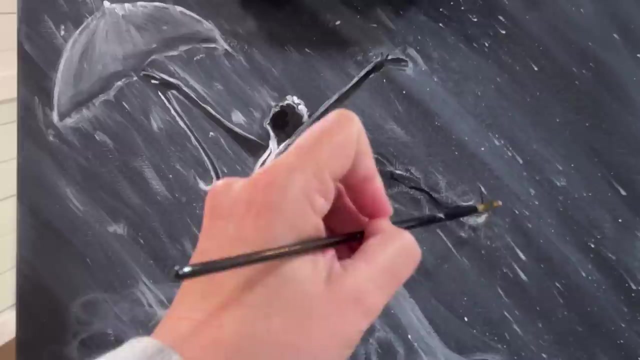 Own to things. You like it, By the way, it's really good. Yeah, yeah, it is, because it's just, I have plenty of time. pick up a little bit of black, add some shadows in there and some contrast to make those highlights stand out a little. 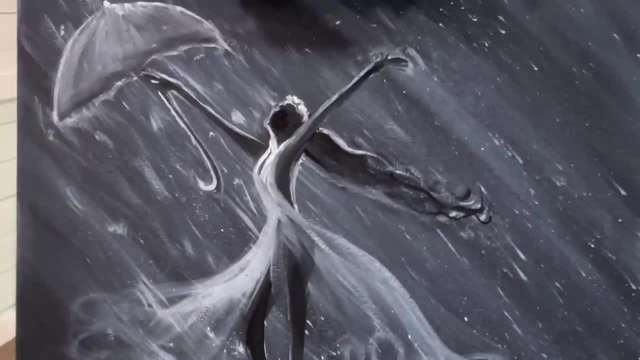 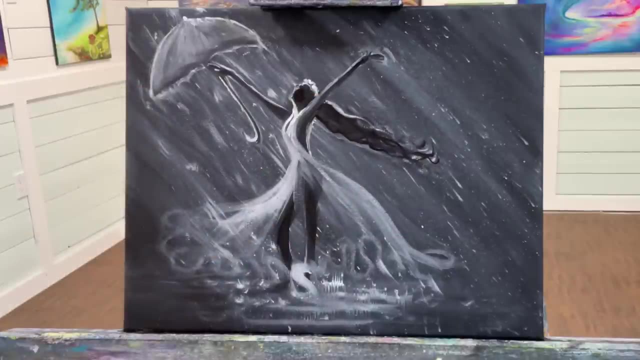 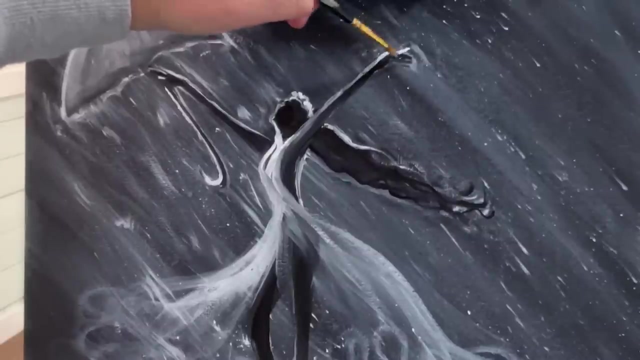 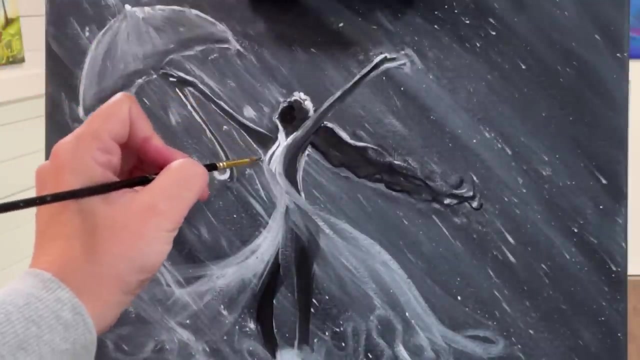 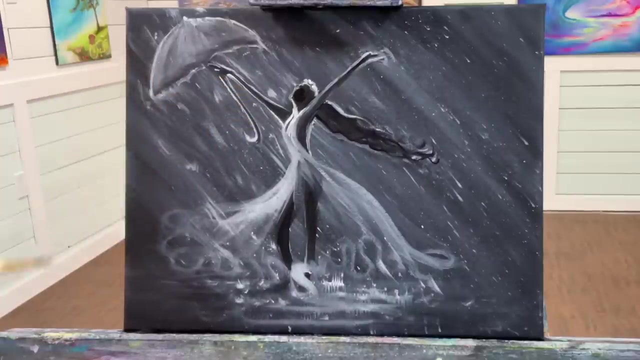 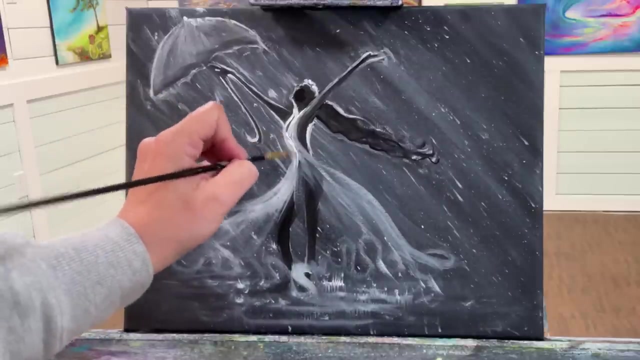 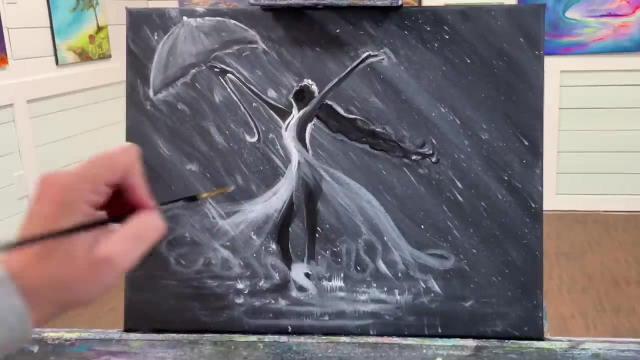 bit better in her hair, remember. it's not about making everything look super accurate and perfectly detailed. it's all about creating emotion, an image that gives you feeling when you look at it. that's what true art is, unless you are an artist that really wants to create realism. photographic types of paintings. 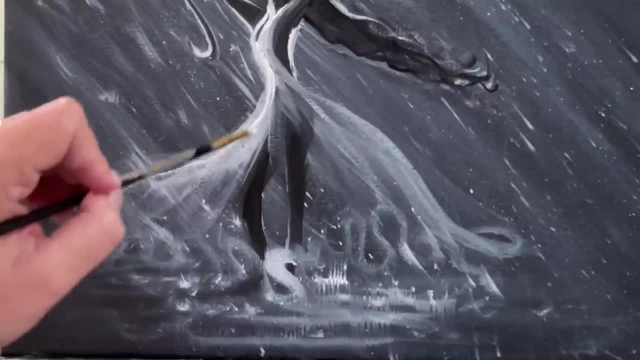 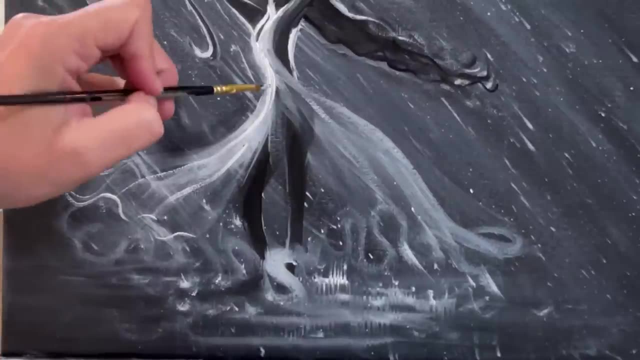 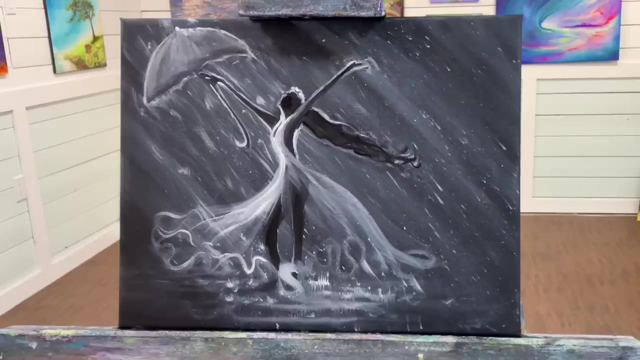 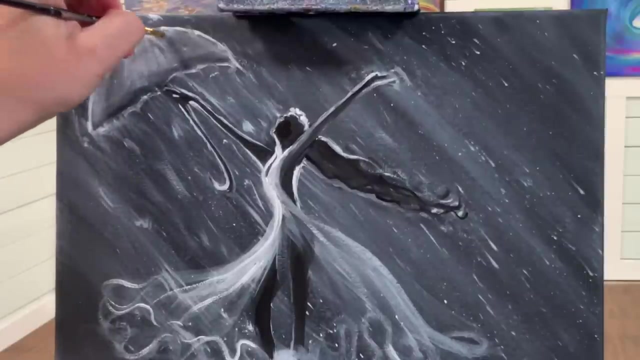 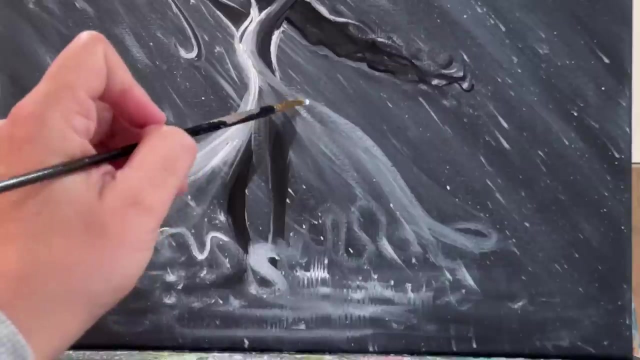 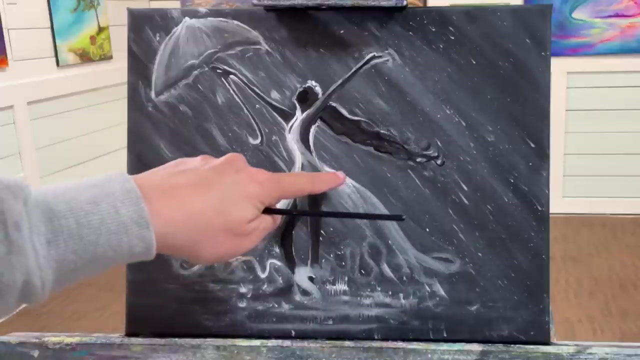 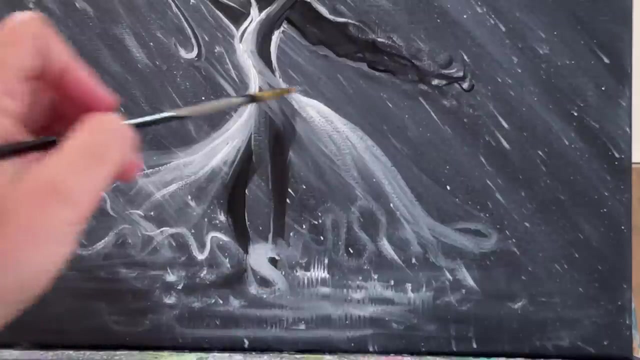 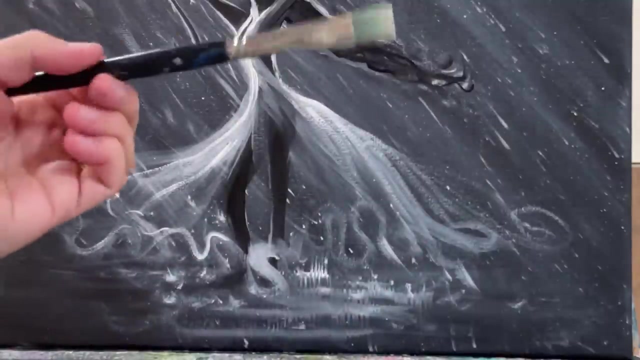 i wouldn't recommend this tutorial for you. you're an artist like that. i'm just taking and sweeping with my brush a little bit more of the white now so i can get some more highlights going. there's going to be some light filtering from behind her. i'm going to use another flat brush now. this is a number eight pro stroke by power krill. i'm going to get my brush a little bit more flat and i'm going to go ahead and add a little bit more of that to my brush, and i'm going to go ahead and add a little bit more of that. i'm going to go ahead and add a little bit more of that. 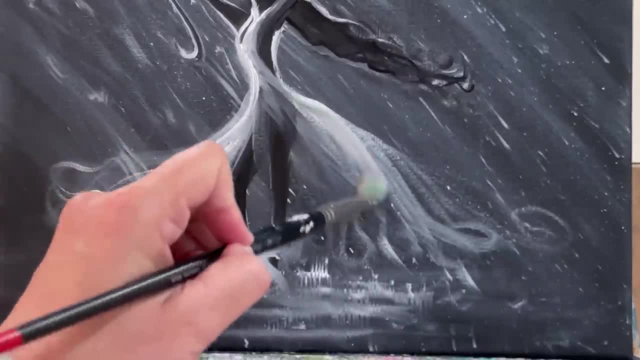 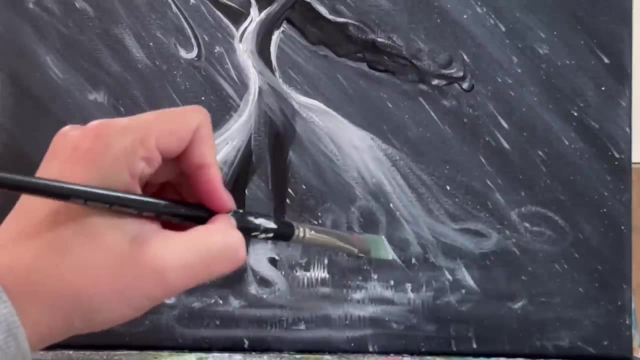 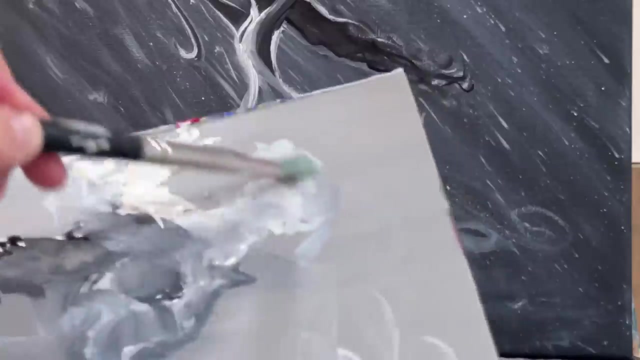 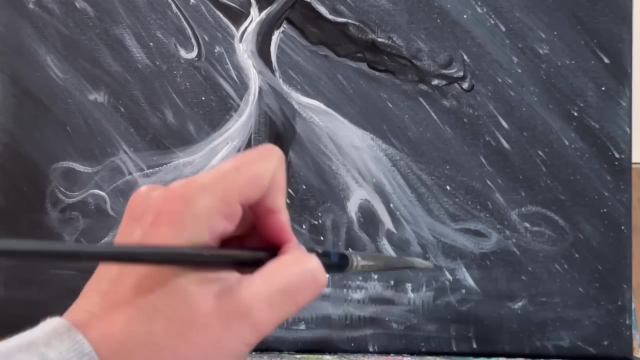 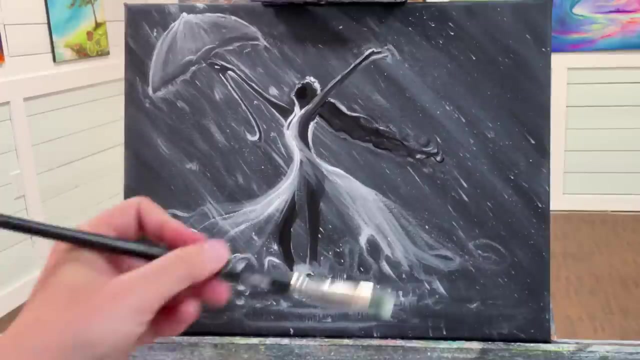 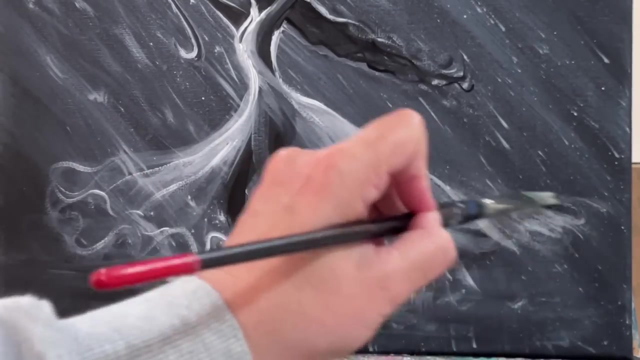 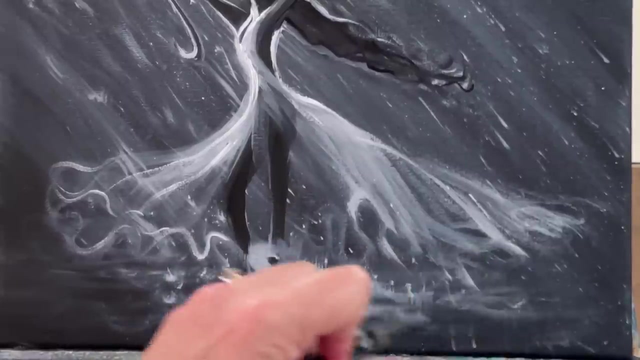 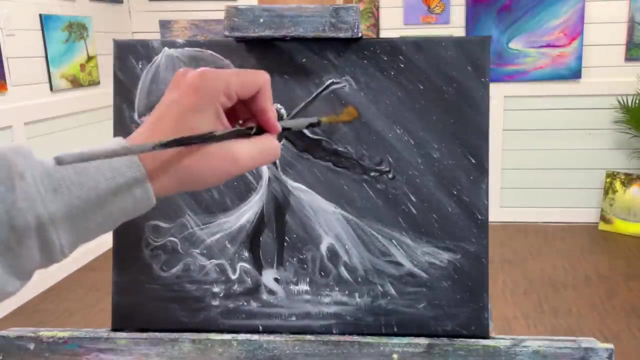 and just start pulling out some of that white. i'm going to pull that shape right there, then get a little bit of water on my brush, line it up, pull, add some reflections down in here. so i'm going to switch over to this. one's a lot softer. 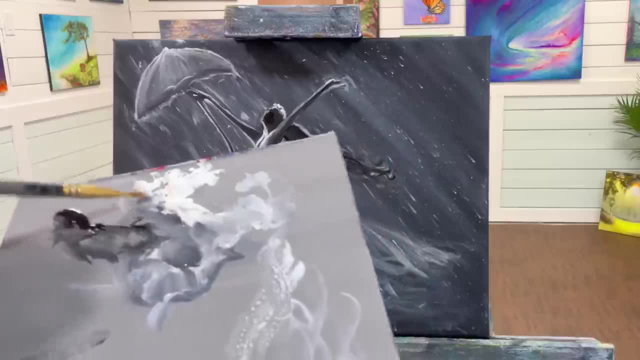 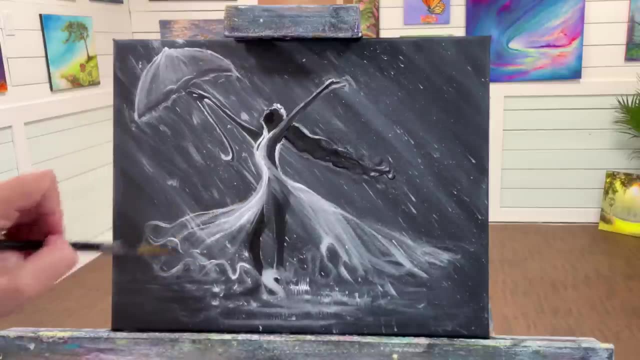 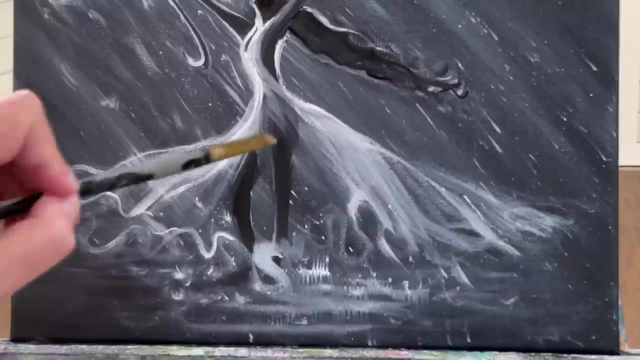 and it'll help me be able to blend better and get more of a flowy effect. so wherever they go up, these ruffles go up, those are going to be on the top and they're going to be the brightest. wherever they dip down is where you're going to have natural shadows, so that's why it's nice to have a dark background. 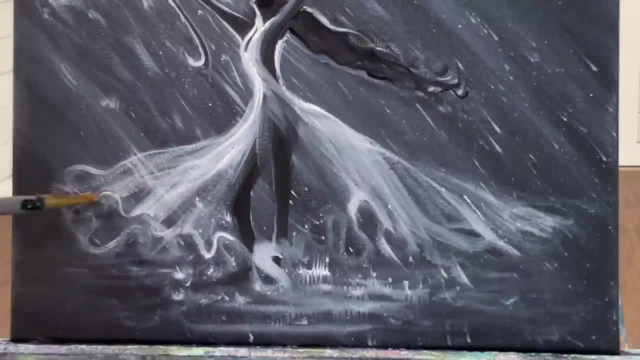 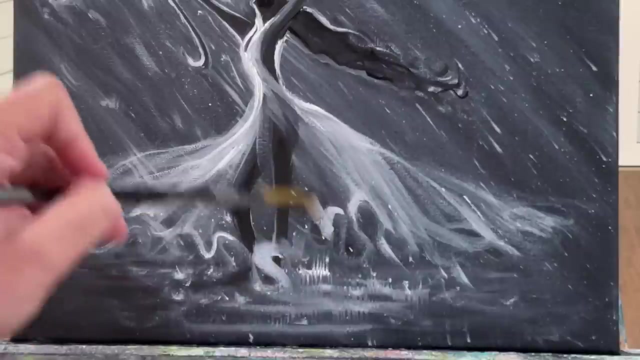 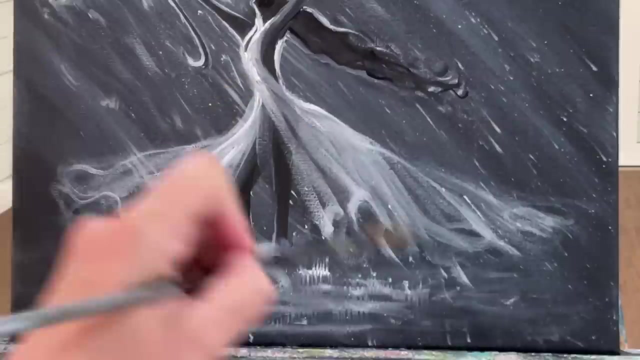 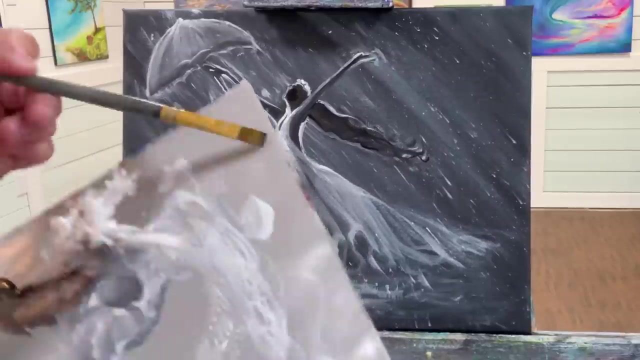 to work on. you get an instant shadow effect. now, of course, we want to create a veil effect, very sheer, look over top and have it kind of twisting around here. you want to make sure her figure is dry, and then i just want to make sure i have. 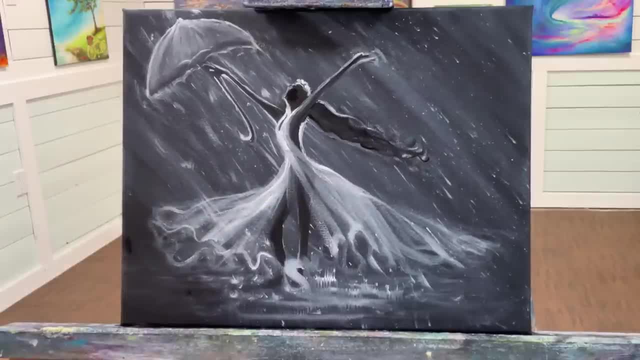 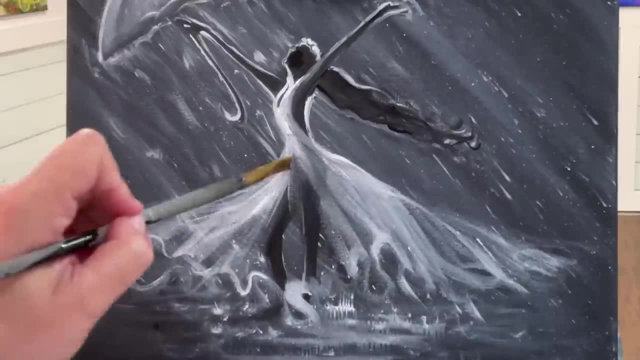 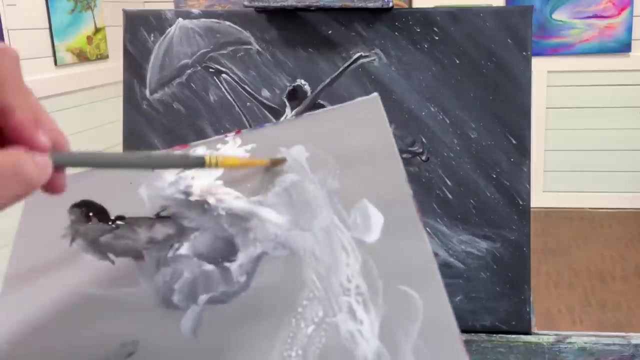 a little tiny bit of water in my brush- definitely not dripping, we won't be able to still see her, her figure, through there. just get a little bit more water on my brush, a little bit, just a hint of that light gray now we'll just do this a little bit more. 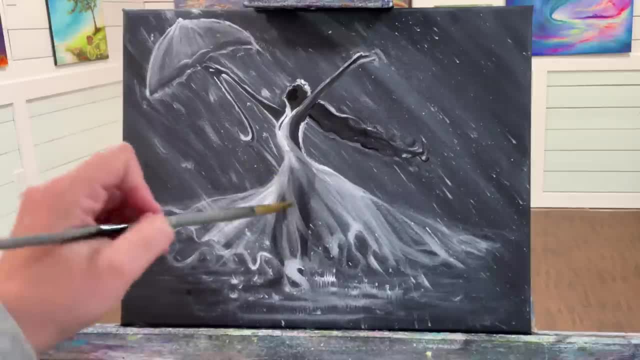 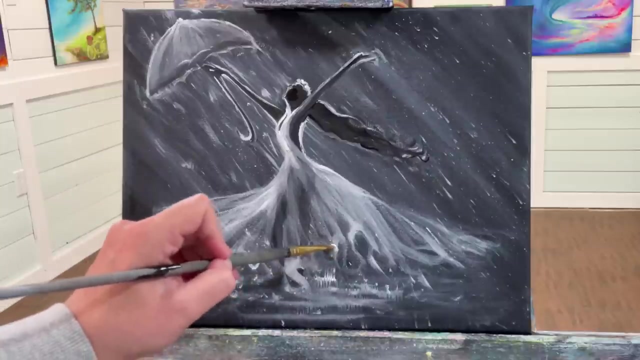 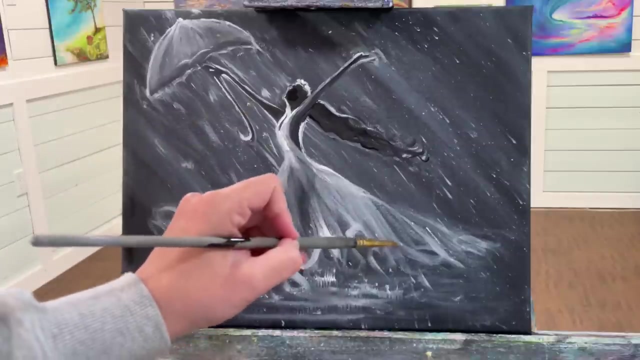 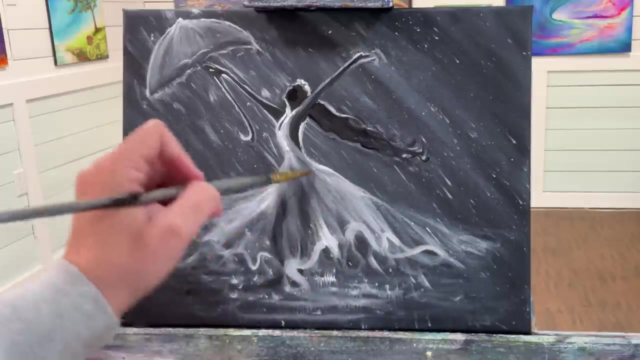 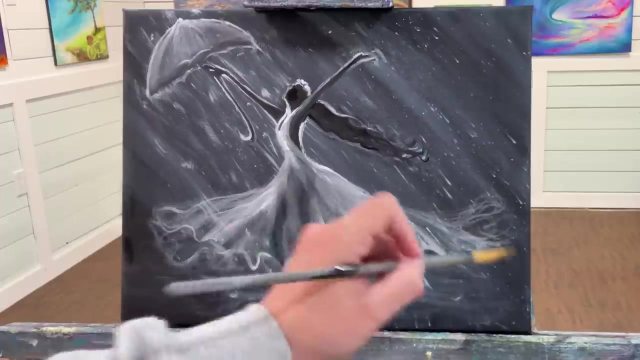 this very carefully, a little bit at a time. let's bring up a little ruffle right there now. when this dries, it's going to be darker and we'll still be able to see her shadow of her figure in there a little bit more. let me just go ahead and just go over one more layer. 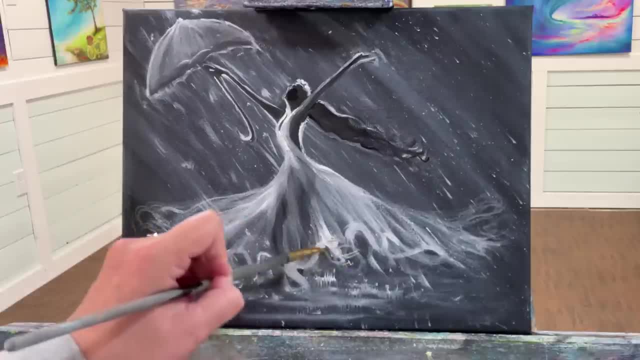 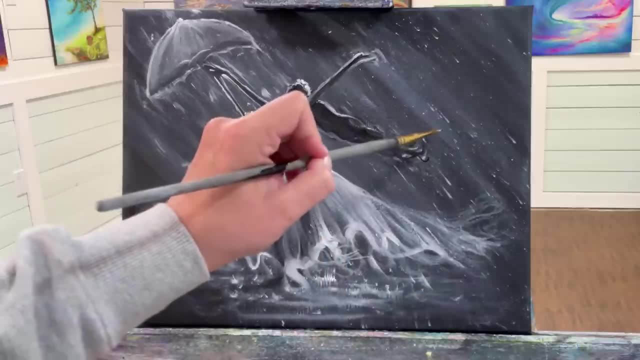 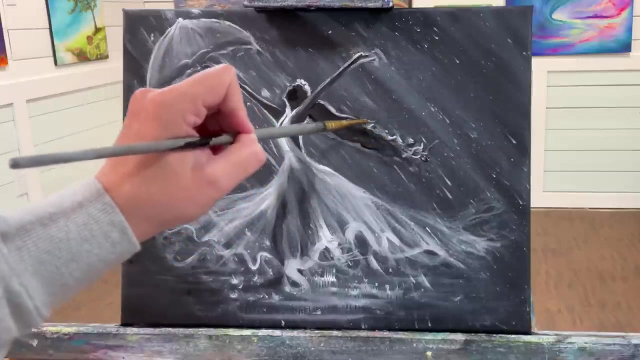 of this one, so you can make it as ruffly and dramatic, exaggerated as you want. have fun with it. it sort of- well, not sort of it really is an empowering image, isn't it? She feels free, She doesn't care that it's raining. 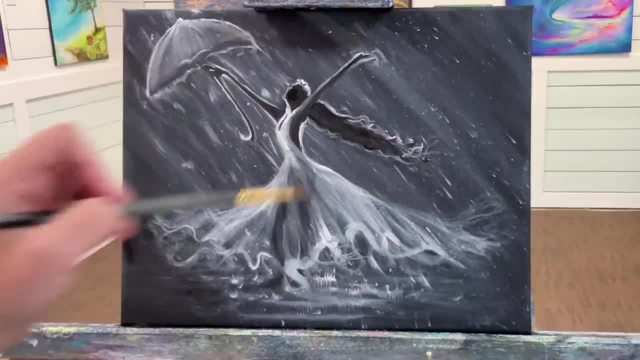 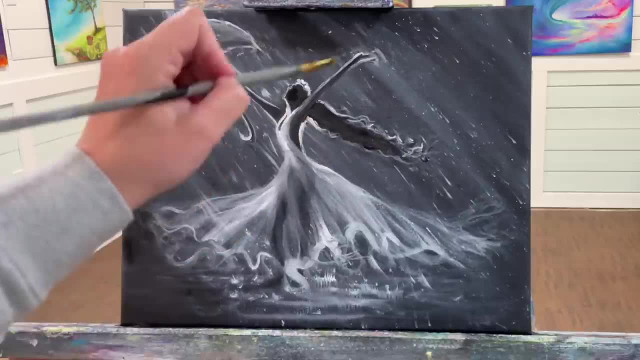 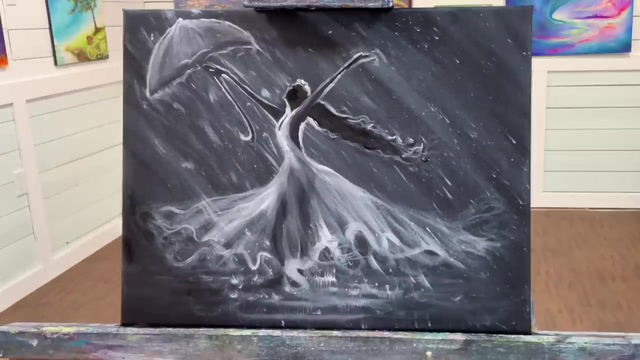 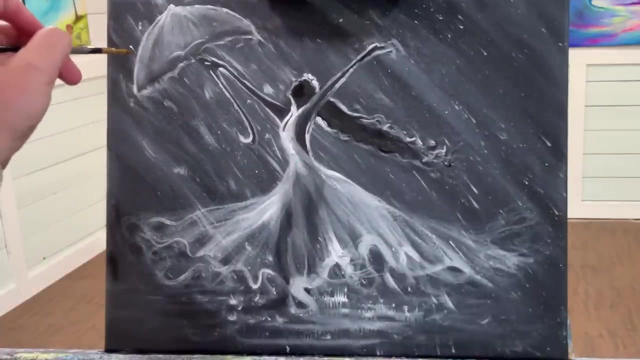 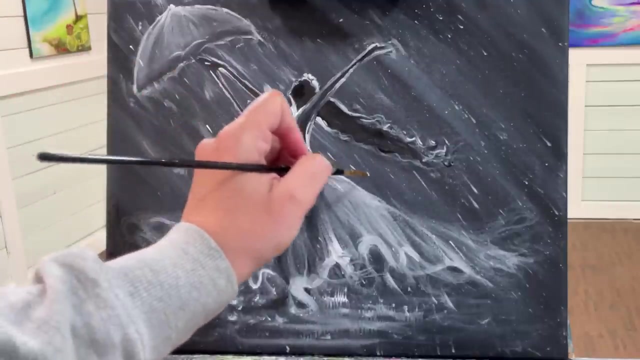 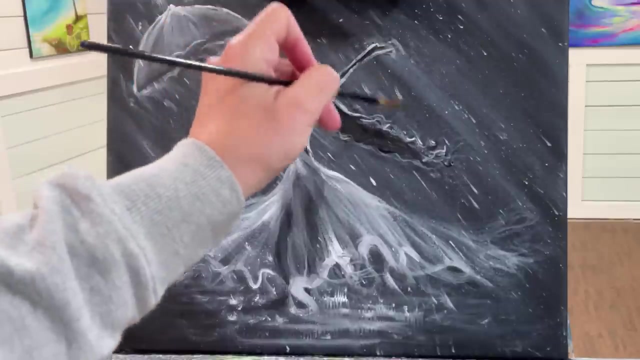 She's enjoying it, Just soaking it all up. We'll stick a light gray through there. Back over to my little round brush And we'll add a few more raindrops. See all the different brushes you can use to create raindrops. 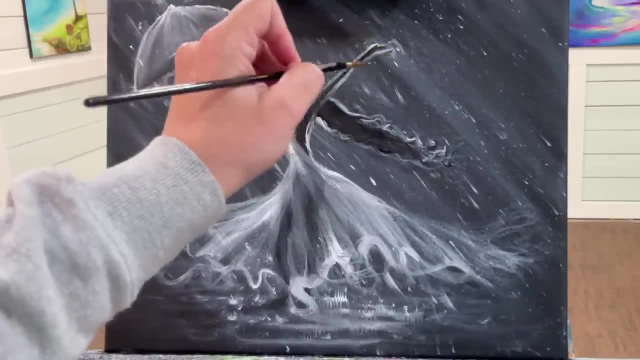 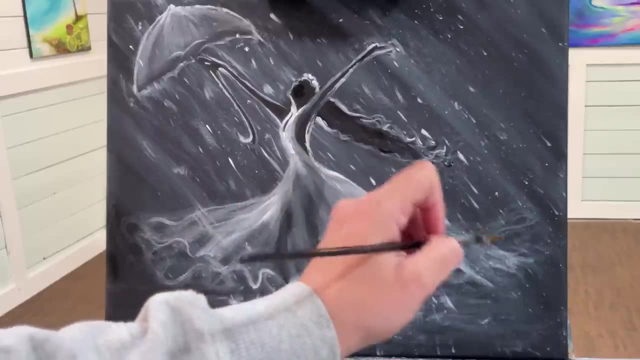 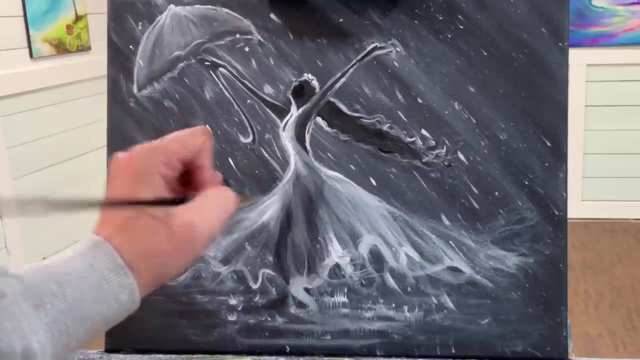 I like to show you guys a few different ways of creating something in a painting. I want you guys to learn as much as you can, And I know not everybody has the same brushes I'm using, So I'm giving you guys alternatives. I'll re-brighten that. 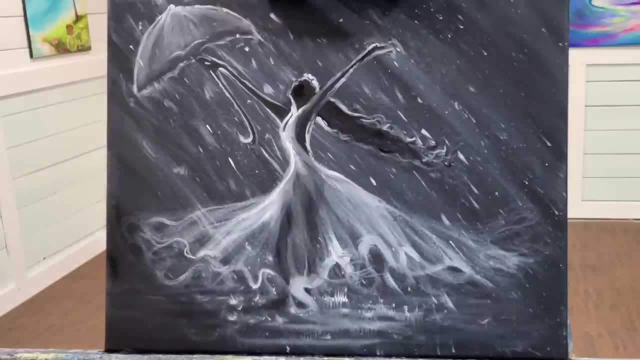 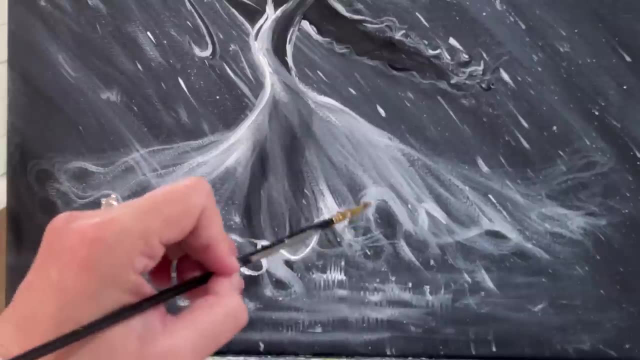 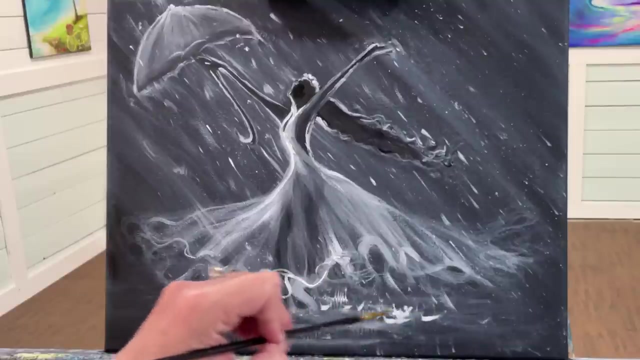 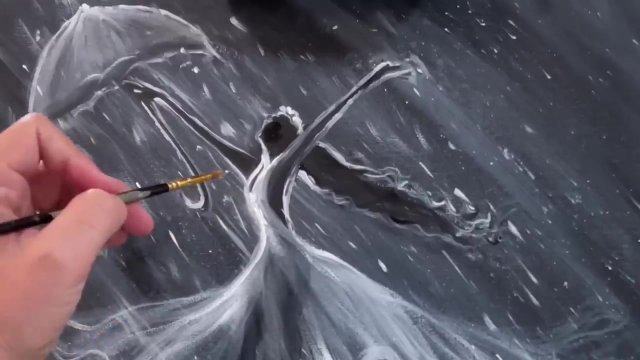 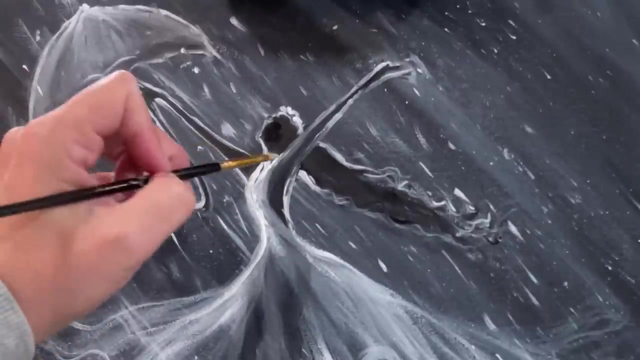 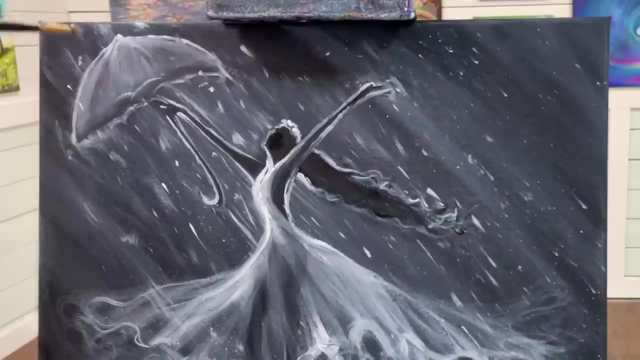 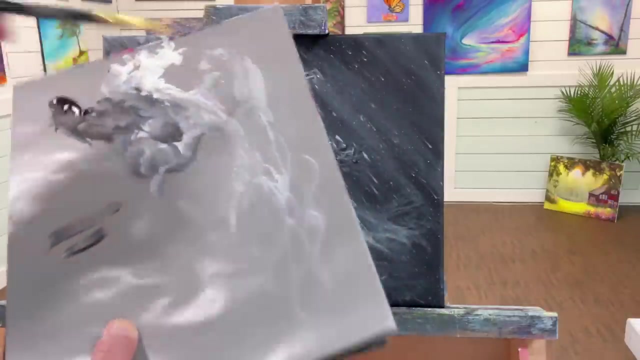 Thank you. I'm going to create a little bit more light here up in the top left corner, Just dry brushing some white. Then what I'm going to do is go back over to my flat brush. A little bit of water in there. 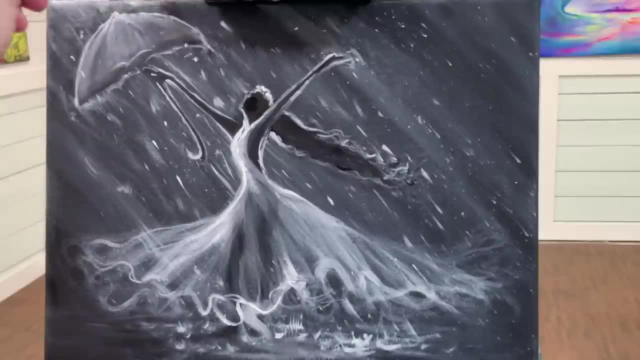 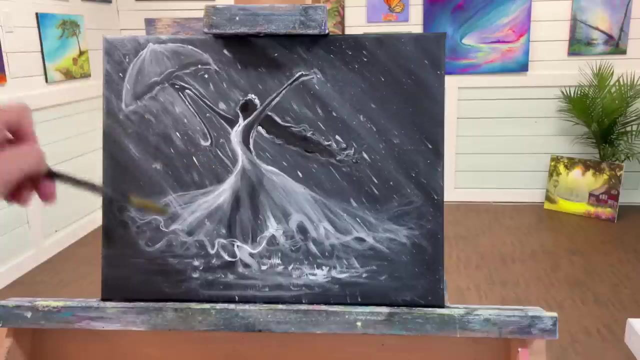 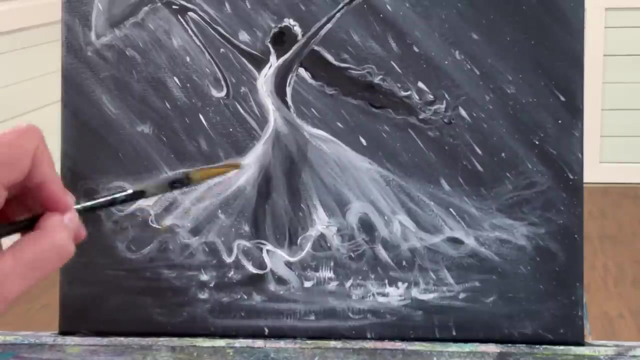 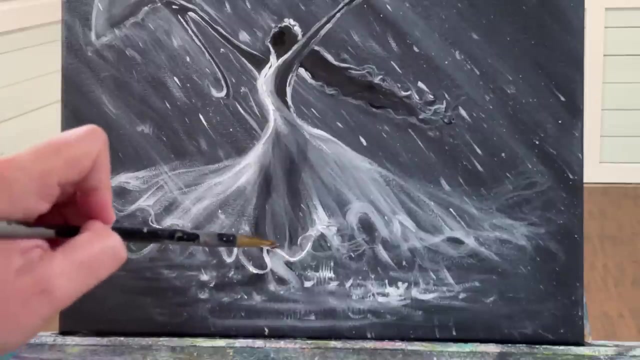 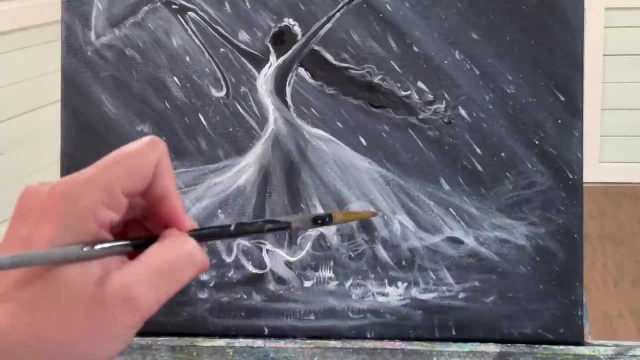 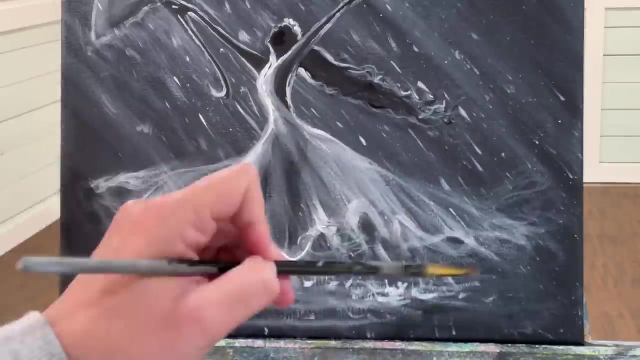 A little white, A little white. I'm just creating some more light. The technique I'm using for her dress is very similar to creating sun rays and how we paint sun rays Now, unlike my lady in red tutorial, which I'll leave a link here for you if you haven't seen that one yet. 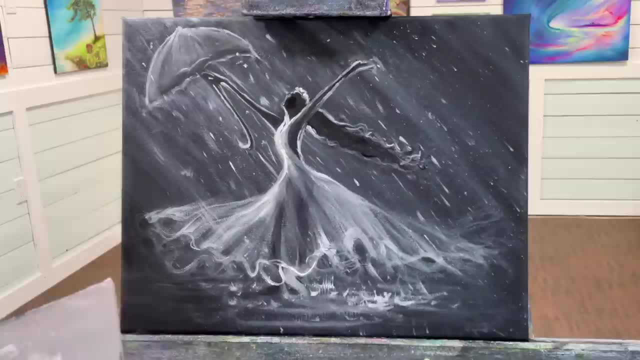 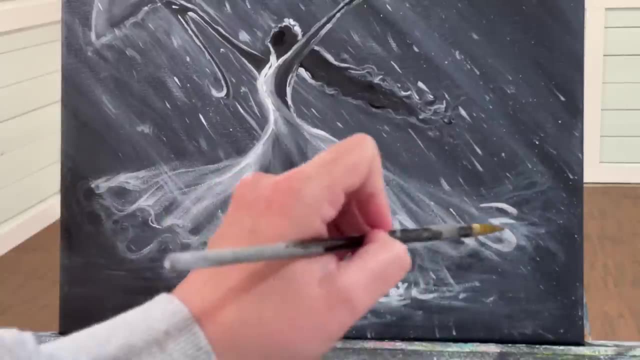 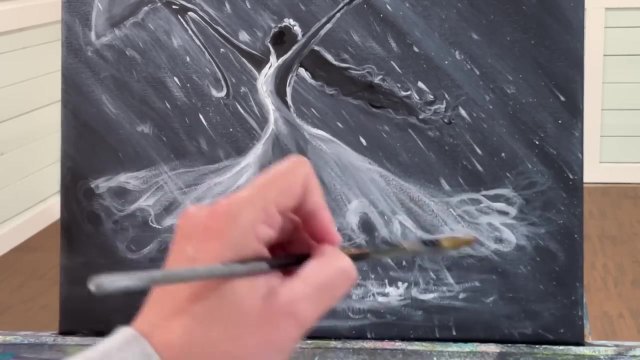 I'm leaving this one black and white. I'm going to leave it up to you guys to add color. if you want to add color to yours, I kind of like this just in black and white myself. If you want to see more colorful dresses for some inspiration, I've got quite a few tutorials in my 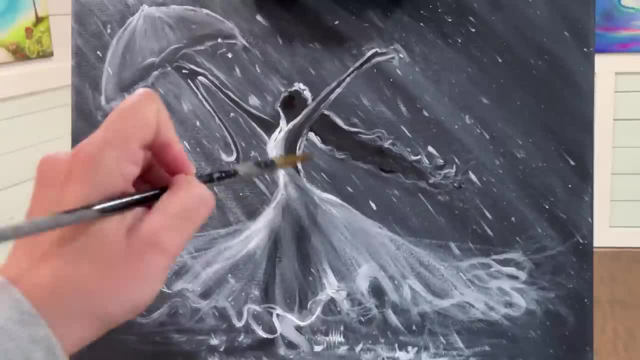 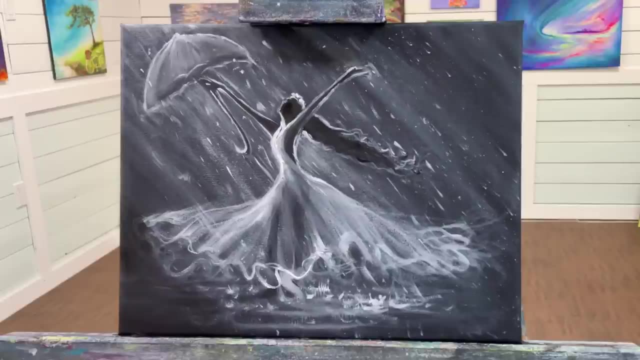 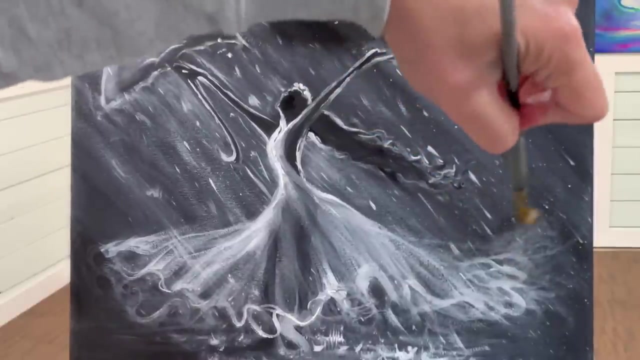 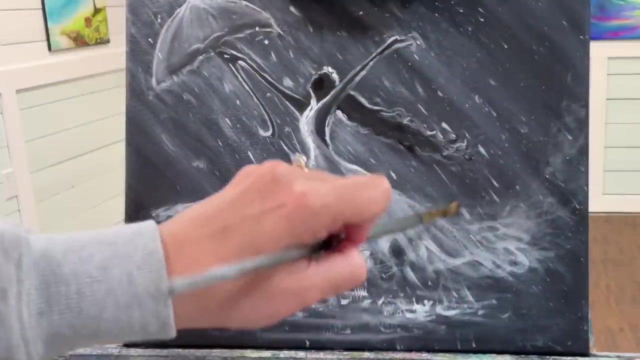 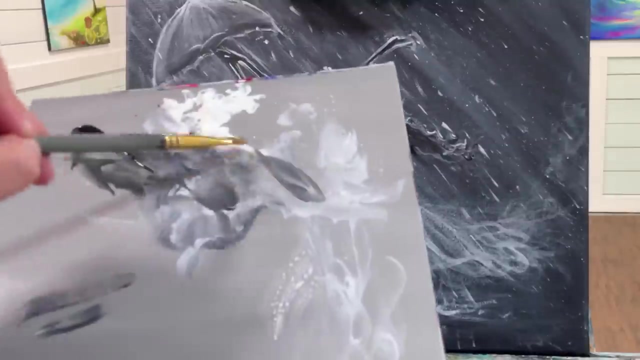 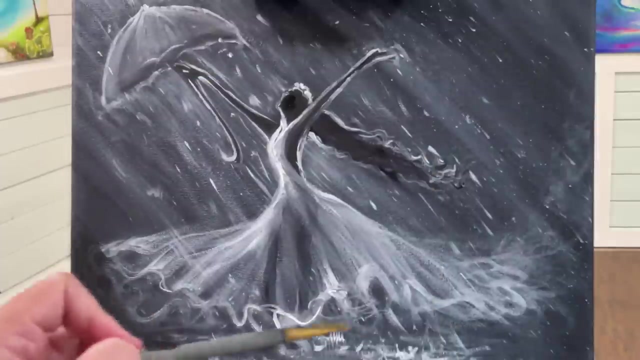 Figures and Portrait playlist. I'm just going to dry brush and scumble out a little bit right here just to soften this area up, Go back in and make some light gray. I want to have it nice and flat and on the end of my brush mainly. 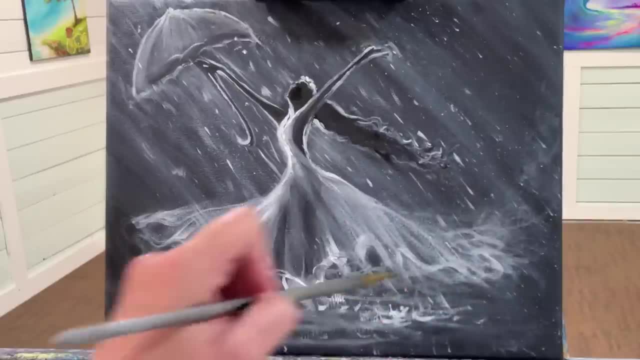 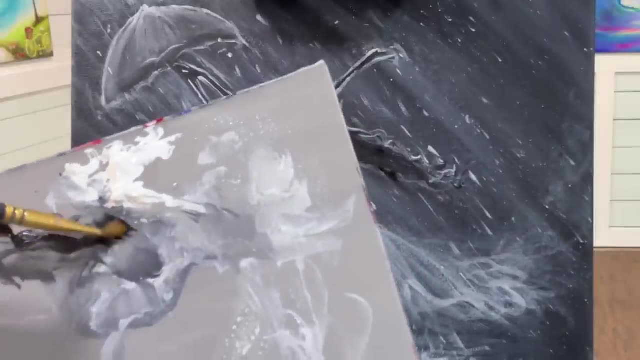 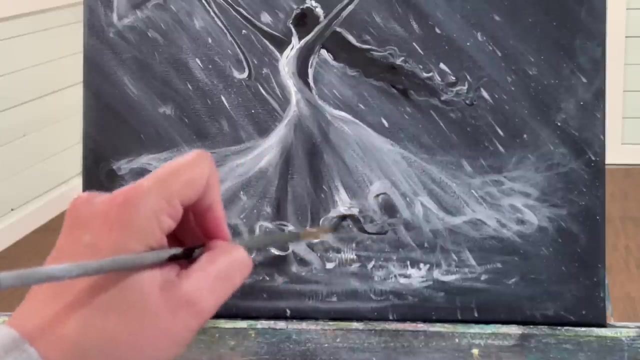 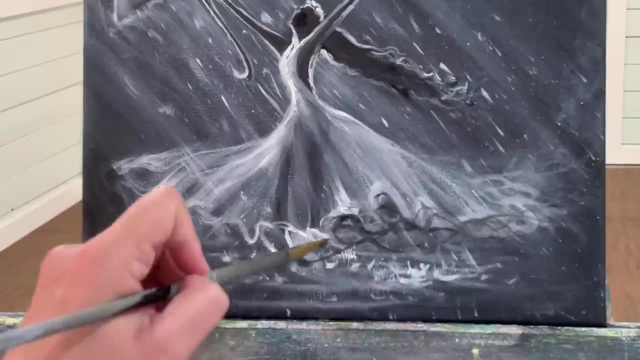 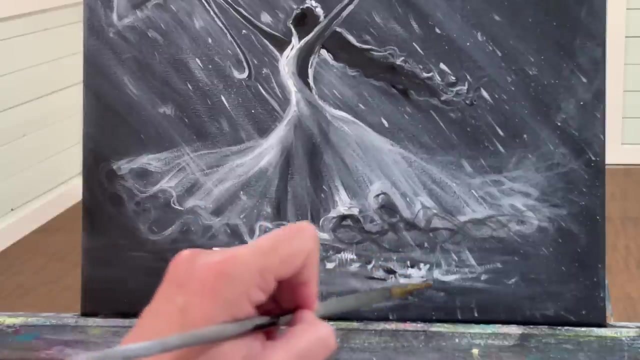 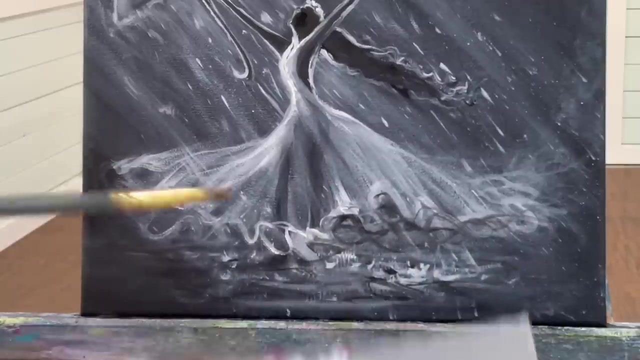 I'm going to create some tight little figure eights here To make some of those stand out just a little bit more. I can come in with a little bit of black, Use a little bit more of the white here, And then I want to create that little reflective. 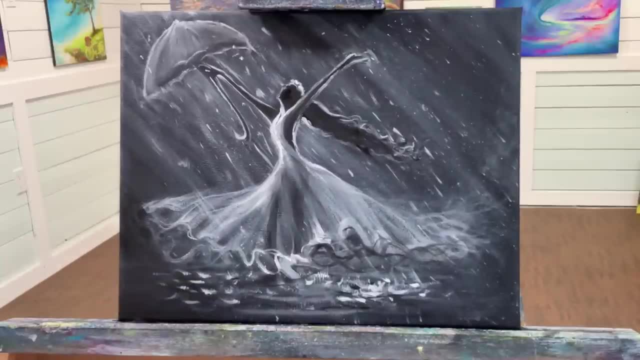 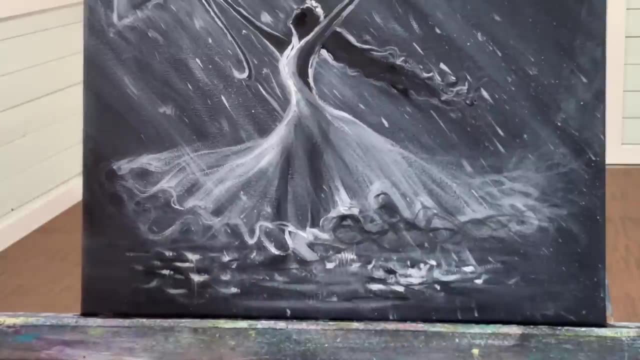 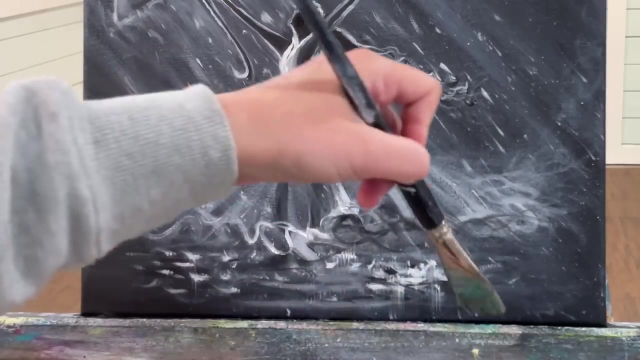 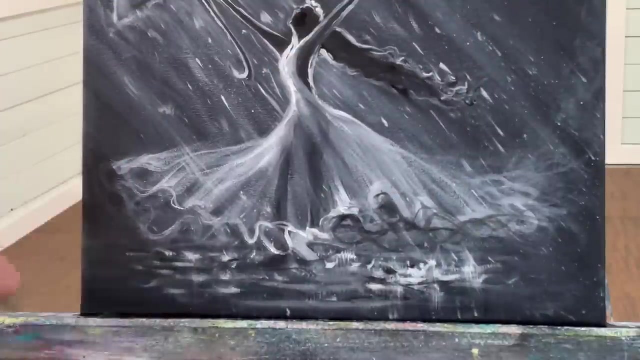 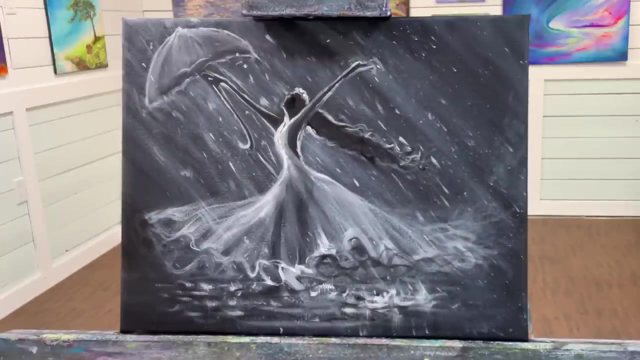 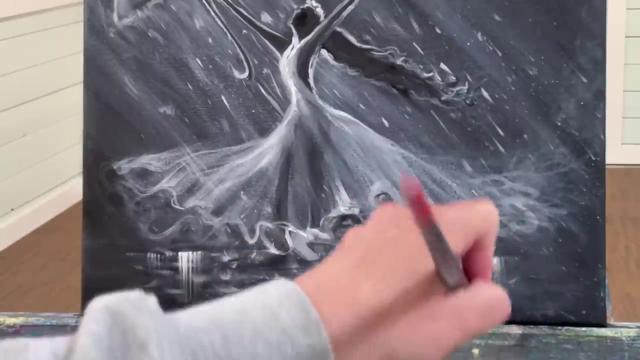 Look that the water has. I'm going to go back to my larger flat brush for this And pull. Remember you can go up the other way as well. Just get a little bit more on my brush. Sorry for the noise. Some fire here keeps. keep hitting my handle on that. 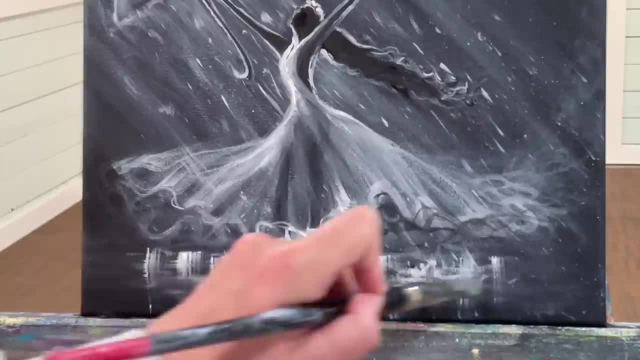 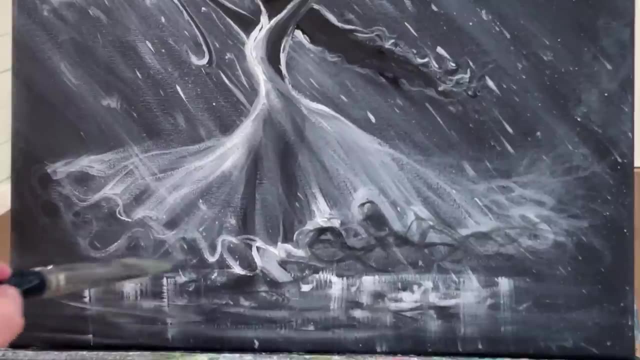 And then sweep across And it looks kind of smeary like water, And then we're going to go back and get a little bit of purple, See Some color. A little bit, Let's go. All right, I'm going to call this one done. 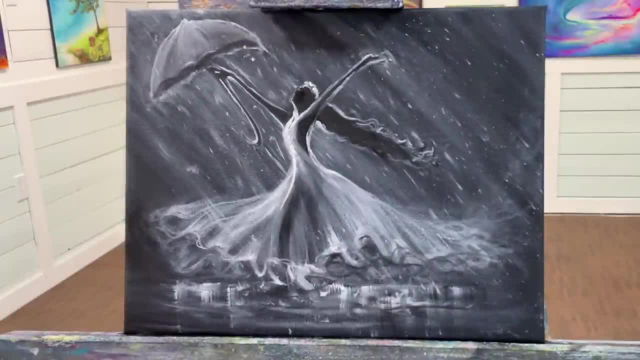 This was so much fun to paint. Hope you guys enjoyed this one and paint along. Don't forget to subscribe to my channel for more. Check out all the links and the full list of colors and brushes canvas below in the description of this video.